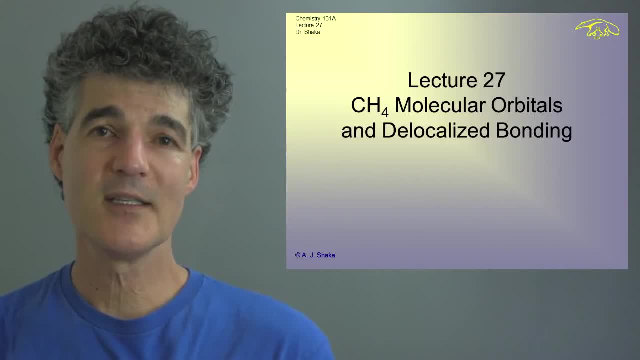 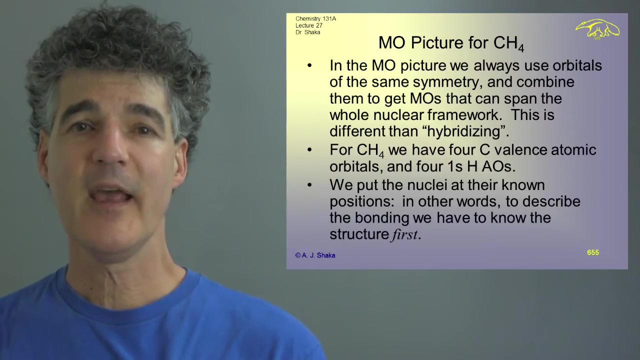 reactions, But occasionally a reaction goes that doesn't seem to behave, and that could be an indication that there's something wrong. Maybe the theory of the lines is falling apart a little bit. Let's talk, then in that vein about more delocalized bonding In the MO picture. we don't make hybrid orbitals, So 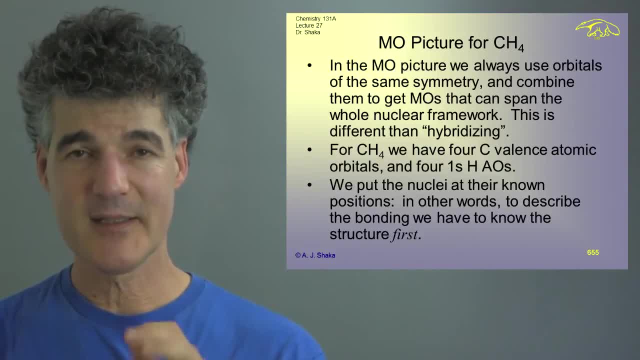 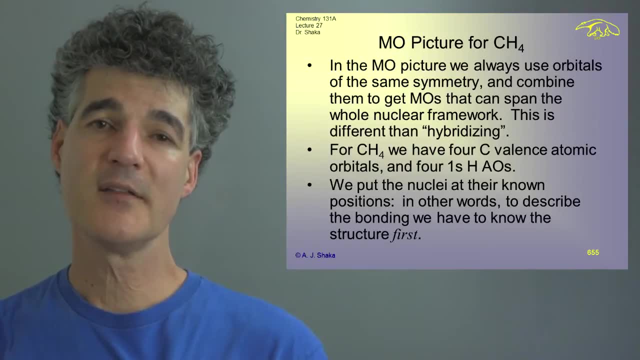 the orbital is used, but it's completely different, So you must not confuse the two. In the molecular orbital picture, what we had said we had to do was we could combine together the molecules that had the same symmetry, similar energy and overlapped in space For a tetrahedral. 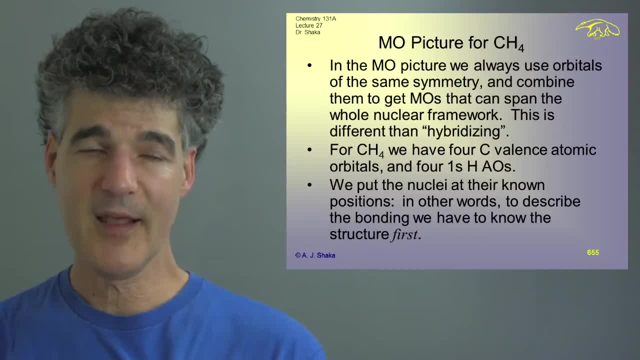 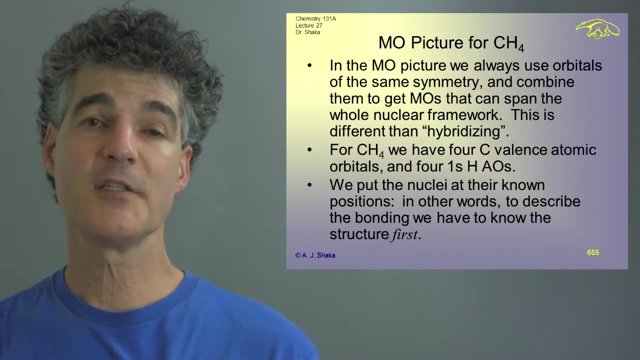 molecule with a central atom like methane. we've got four carbon valence atomic orbitals: the S and the three P's. We have to know the structure, Why? Well, otherwise we'd have to move the things around and calculate the energy as a function of R and R2 and R3. And 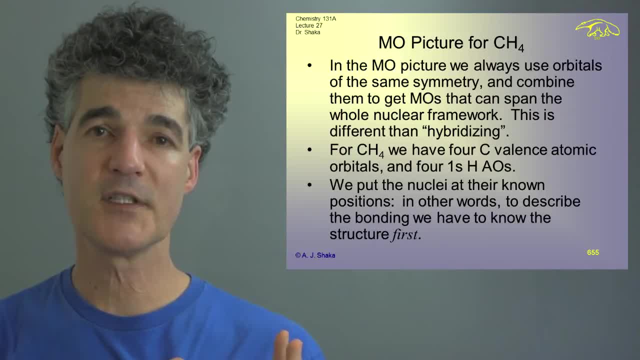 we already know the structure. It's tetrahedral. What we want to understand is not the structure, so much We want to understand the bonding. How is it working? What's going on? So we assume we know the structure. It's the same structure as Pauling's, But the description. 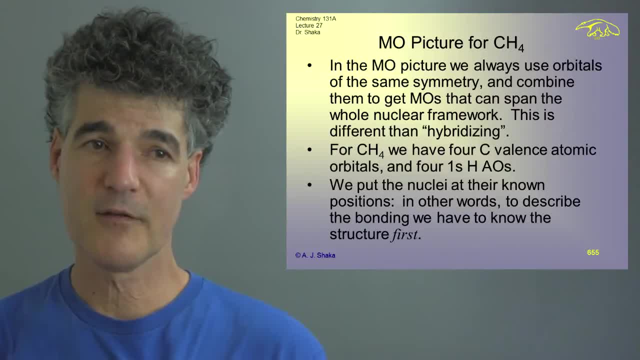 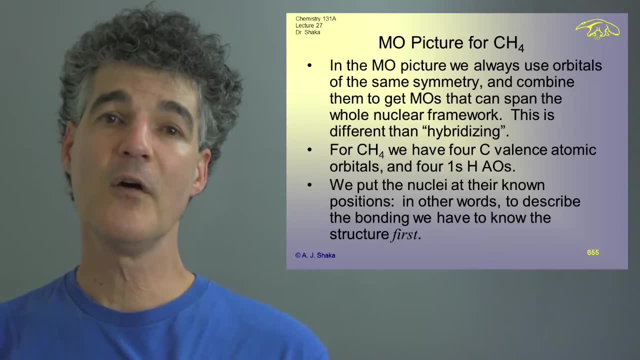 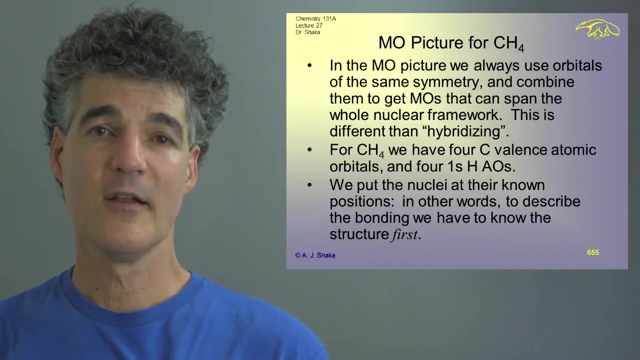 of the bonding is going to be different, And that's the thing that we're going to focus on. So in the MO approach, you have to know the structure first. If you don't, you have to search through all possible structures. If you're doing that, that is a very, very, very 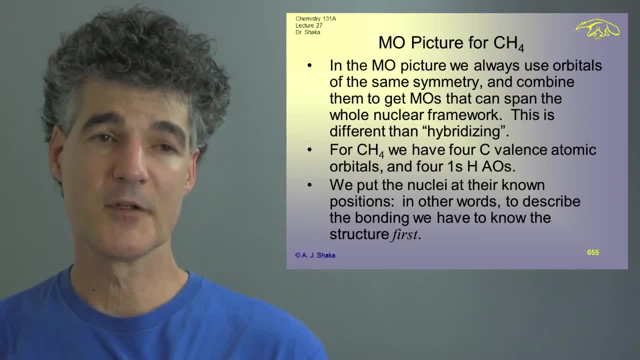 long-winded and intensive calculation, although sometimes people do it just to see what might be the most stable structure. if there's no experiment or it hasn't been made, Let's put our hydrogen atoms at the corners of the same cube that we had before. 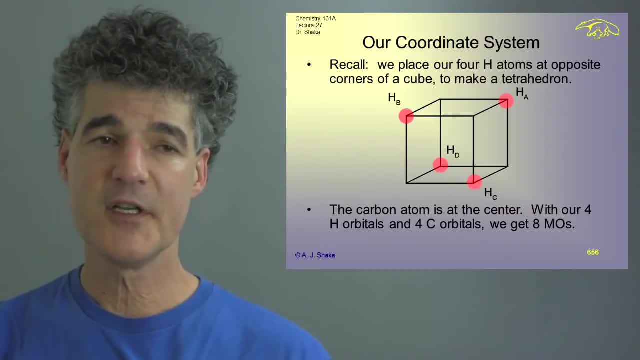 H A, H B, H C and H D. And let's see what we're going to do with these four. The carbon is at the center And with our four hydrogen orbitals and our four carbon orbitals, 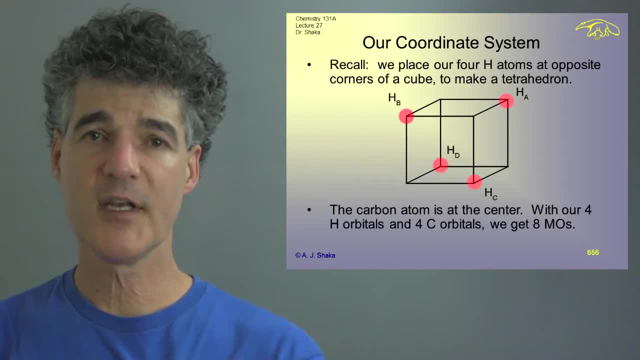 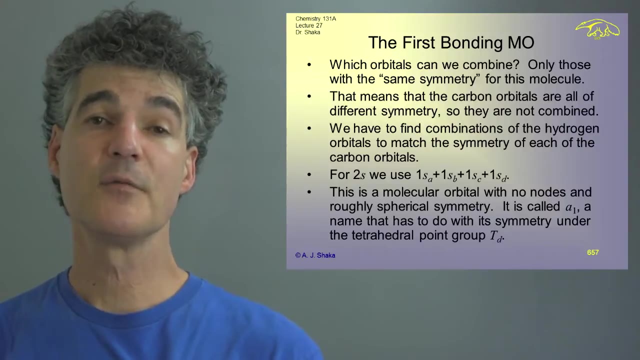 we get eight molecular orbitals Because, recall, in the linear combination of atomic orbitals rubric we have the same number of orbitals at the end in terms of molecular orbitals that we started with. Okay, now the question is: which orbitals can we combine And the 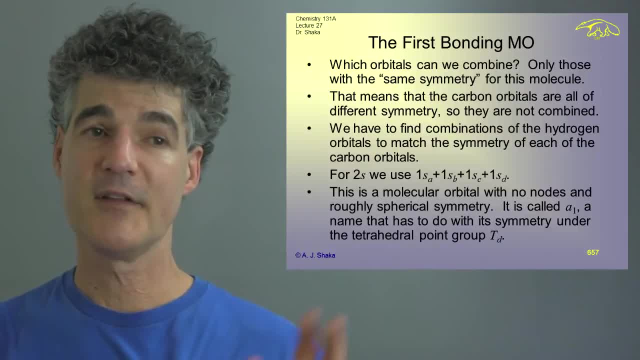 answer is: rule two said they have to have the same symmetry for this molecule, And what that means is that we cannot do what Pauling did, because we cannot combine the carbon 2s and the carbon 2pz or the other two p's because those have different symmetry. They're 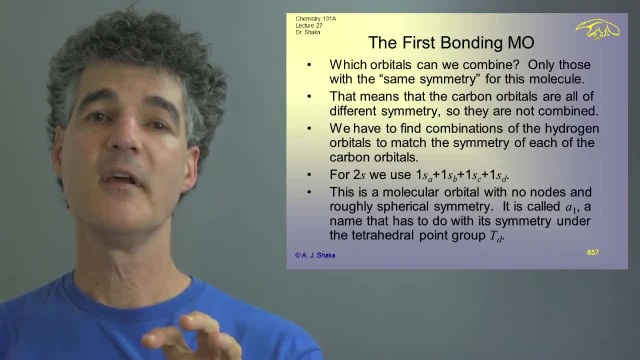 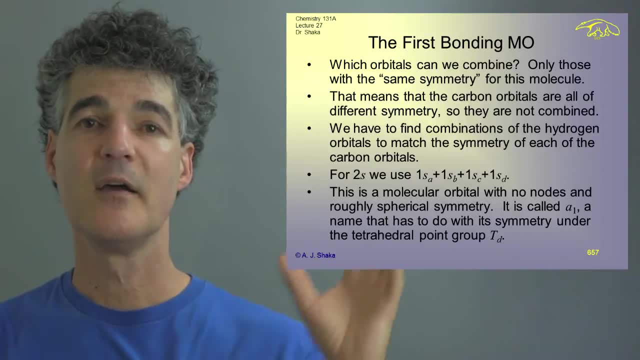 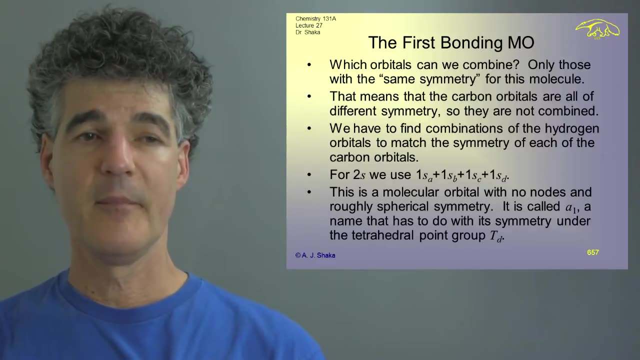 identical. Therefore, if we want to consider the 2s on carbon, we cannot combine it with any of the other atomic orbitals on carbon. We have to instead combine it with combinations of the hydrogen orbitals at the four positions of the cube, And that's completely different. 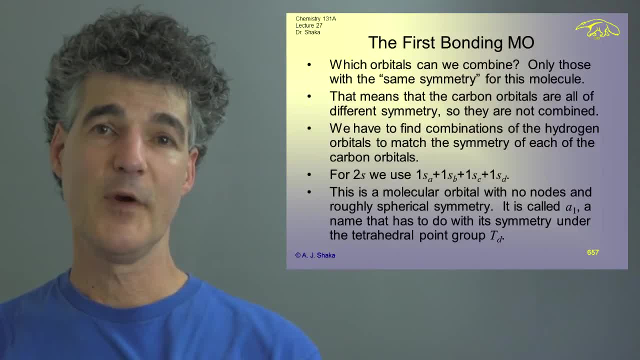 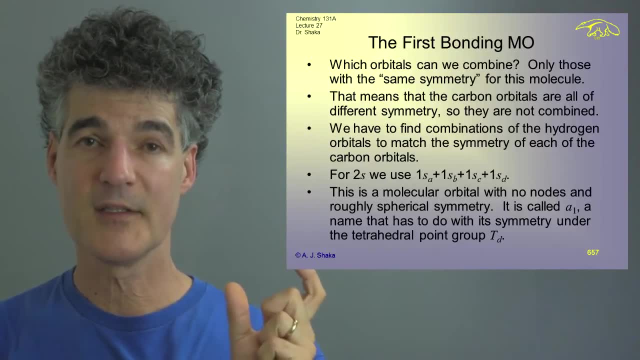 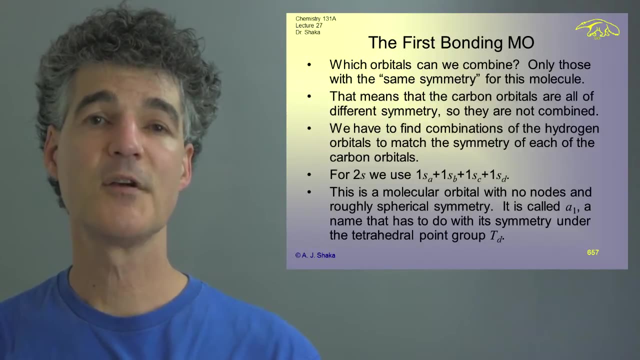 then, because now we won't necessarily end up with four identical lines in terms of four localized bonds. We will end up with a tetrahedral structure. that's for sure, because we started with that, But our description of the bonding will be different. Now the game is this: We 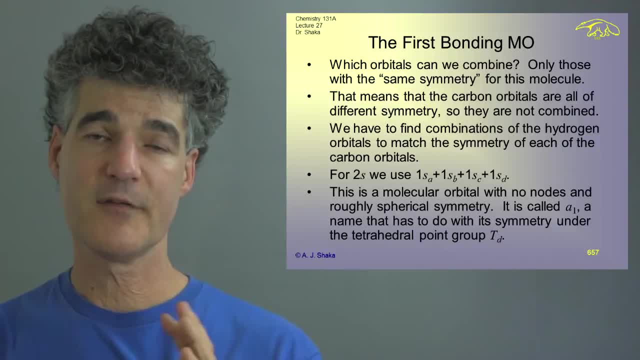 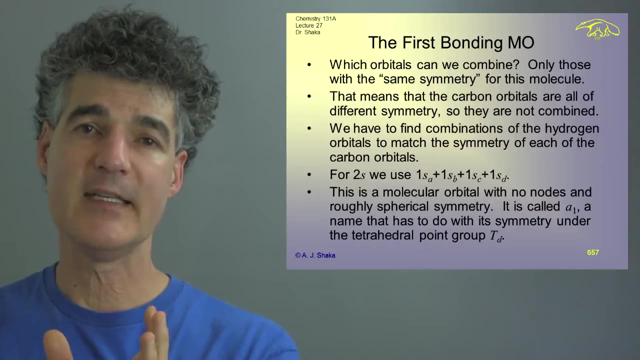 have the carbon orbital. Each of the four of them has different symmetry. We have to combine the four hydrogens so that they have the same symmetry as the carbon orbital. And that's pretty easy to do, because if the carbon orbital is a big fat round S, then we're going. 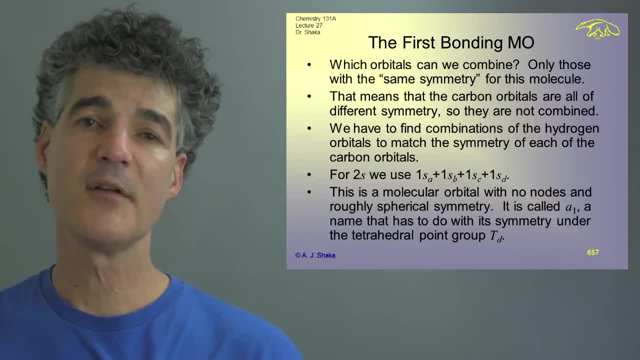 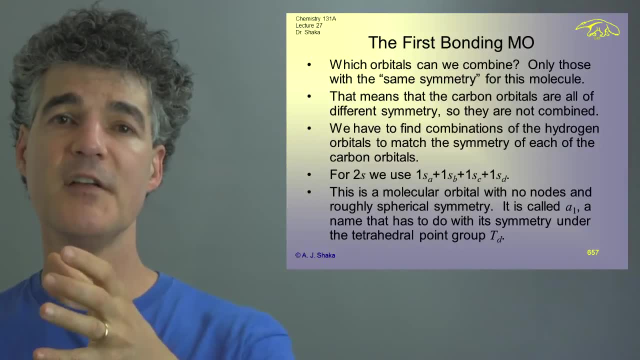 to have the same symmetry as the hydrogen orbital. And if the carbon orbital is a big red, then that means that these guys have to be as round as possible, So they should just all be red And that should be one of them. And if the carbon orbital changes sign. 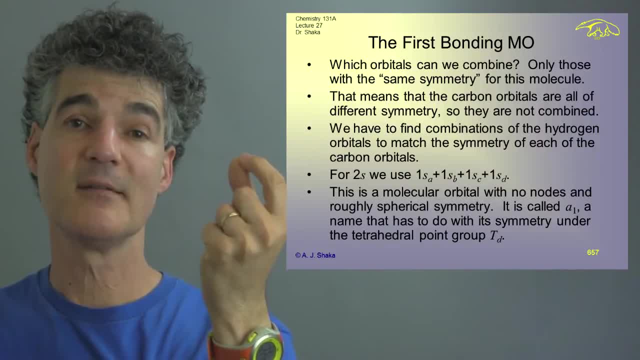 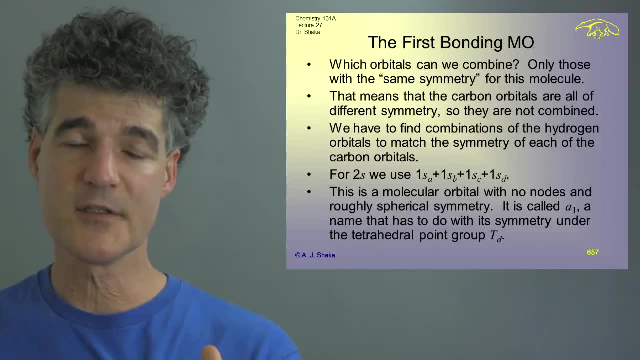 like it's plus here and minus here. well, we've got two hydrogens on the top of the cube. they should be plus Two hydrogens on the bottom of the cube, they should be minus, and so forth, And so there's a combination of hydrogens that goes perfectly with each of the four. 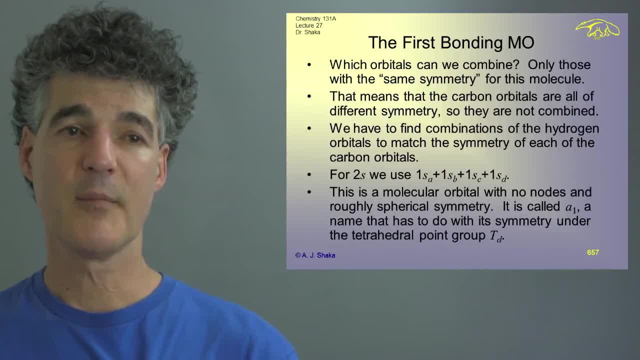 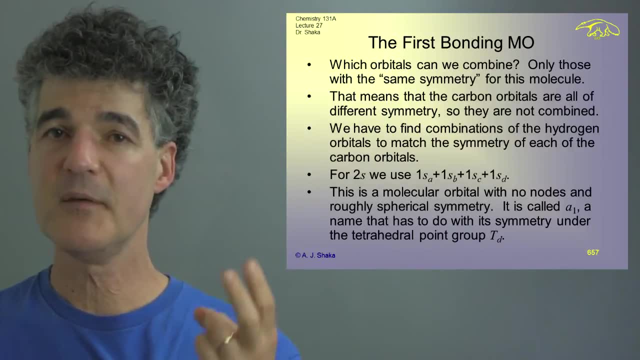 of the five elements. Thank you, Dr. Thank you Dr. Thank you Dr. Thank you. 4. combination on the carbon. and that's how we're going to do it. So for 2S, we use 1SA plus 1SB plus 1SC plus 1SD. 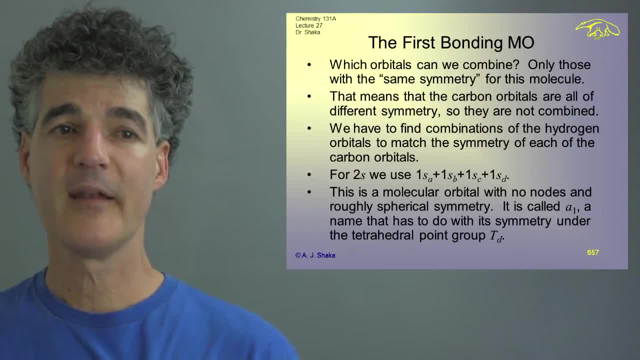 all of them as round as can be. And this then, if they're all red, the 2S is red and all these guys are red. this makes a gigantic orbital with no nodes that goes around all the nuclei and has roughly spherical symmetry. 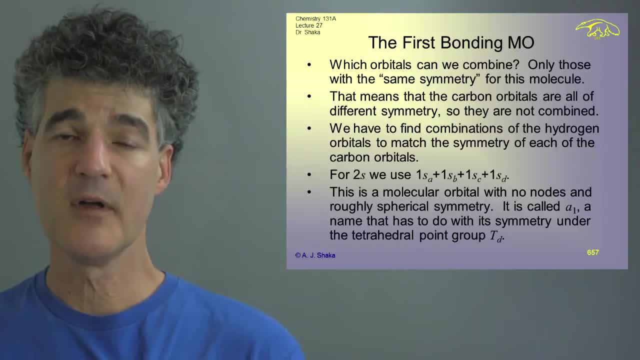 And it's called A1,, which is a symmetry label that lets a spectroscopist know what the symmetry of the molecular orbital is. And that name- A1, has to do with its symmetry under the tetrahedral point group TD. that you'll learn. 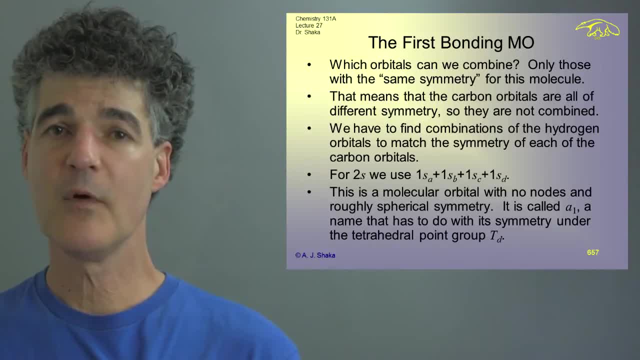 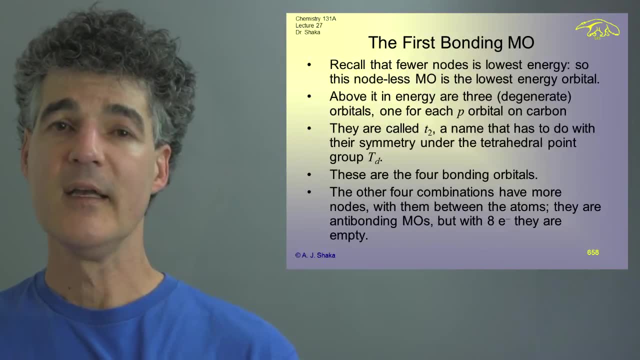 about later in the course. For now, we're just going to treat A1 as a label that tells us which orbital we're talking about. Remember that less nodes is lower energy. and so we've got this big red thing with this big fluffy thing. 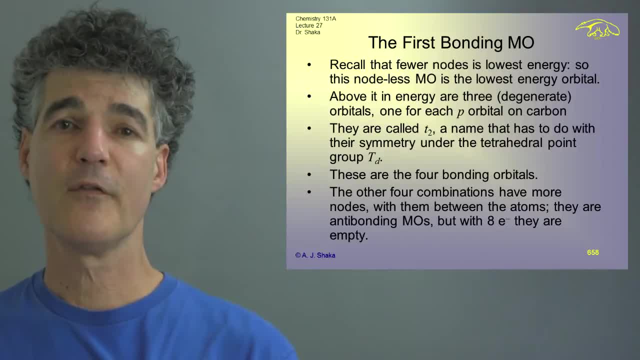 sort of looks like a teddy bear with no nodes. Therefore, A1 is the lowest symmetry. That's what we predict Above it, then are 3 degenerate because they're related by symmetry orbitals and there's one for each. 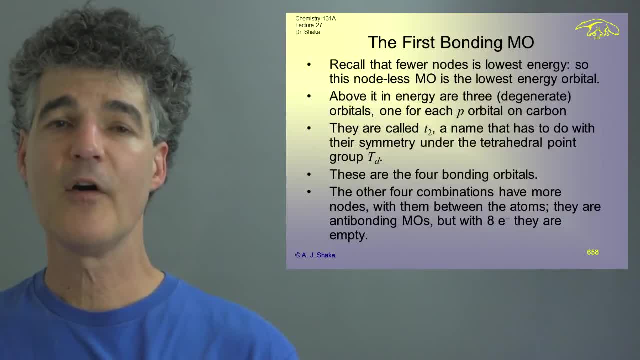 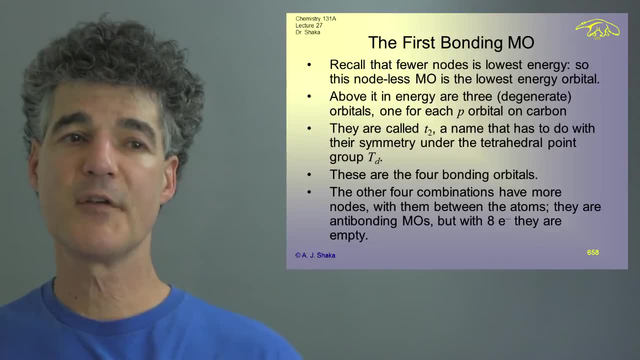 of the P orbitals. The P orbitals on the carbon atom And those 3 are called T2,. T means 3, a name that has to do again with their symmetry under the tetrahedral point group. The 1 and 2 have meanings, but I don't want. 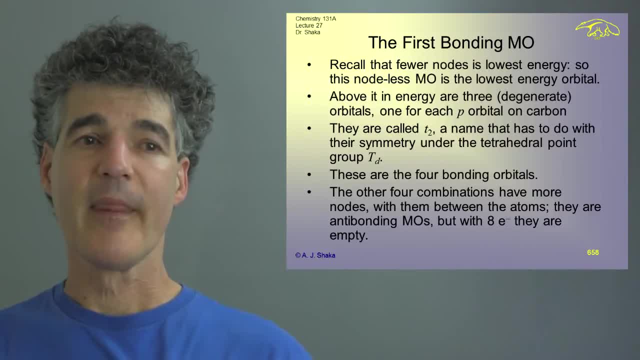 to go into the exact meaning now, These are the 4 bonding orbitals and they are not the same, but there's 4 of them and they still predict an exactly tetrahedral structure. Not surprisingly, because we started out with an exactly tetrahedral structure. 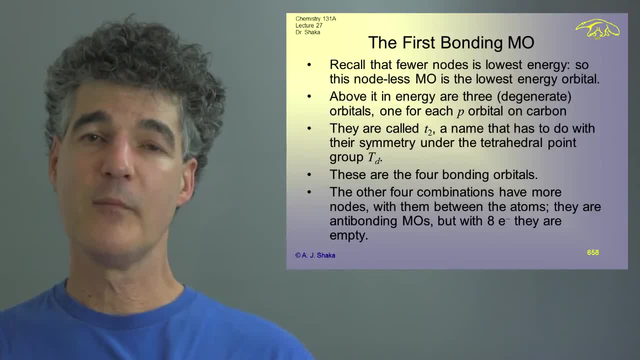 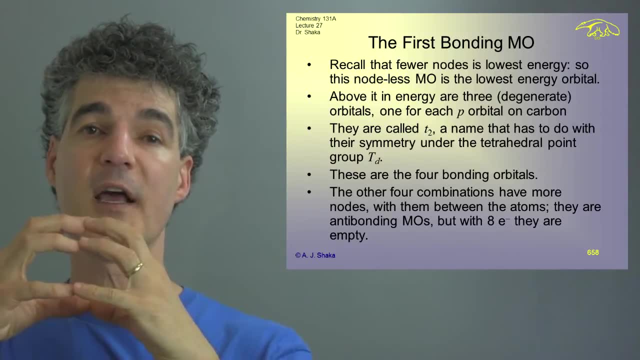 The other 4 combinations have more nodes. I could take the S as red and I have to have some of the same symmetry, but I can pick them all blue. Now that's a disaster, because now there's nodes in between the 2 nuclei. 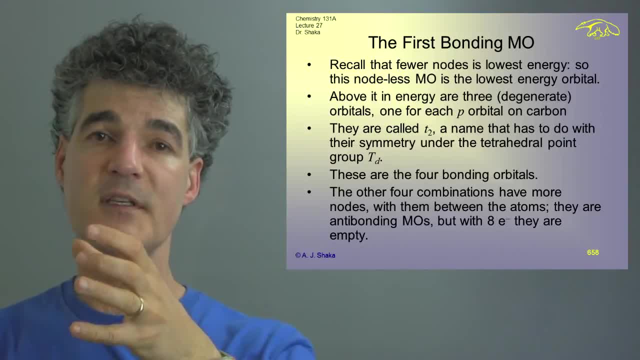 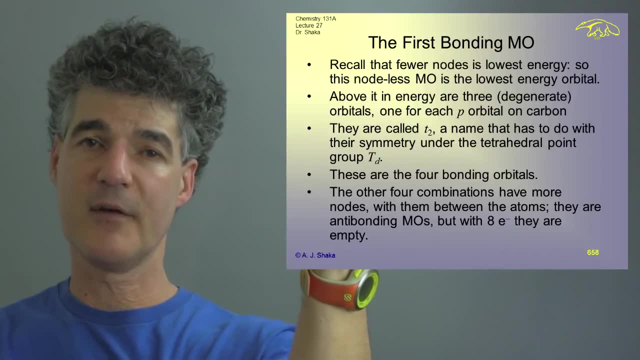 So that one's no good. And likewise I could pick the PZ with red on the top and blue on the bottom, And I could perversely pick these 2 guys to be blue rather than red, and then there would be destructive interference. 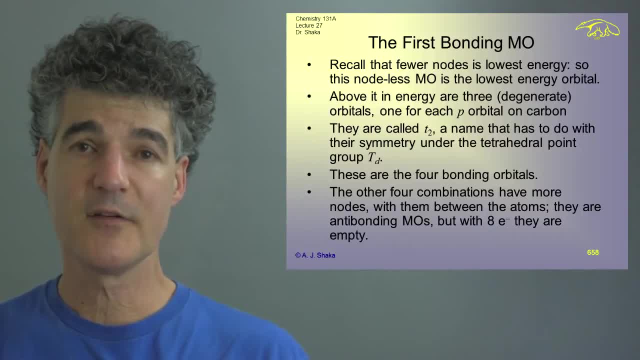 And, again, that would be a very high energy solution. Therefore, we can easily see that there are 4 bonding orbitals. So there's going to be 4 bonds, good, And there's 4 anti-bonding orbitals. 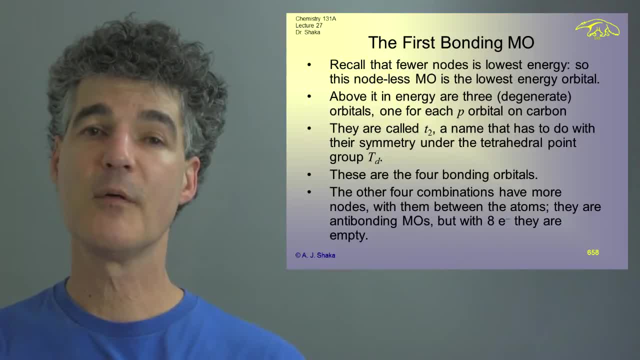 And since there's only 8 electrons, the 4 bonding orbitals are filled and the 4 anti-bonding orbitals are empty. So that's a disaster. Thank you, Thank you, And that's almost always the way it works. 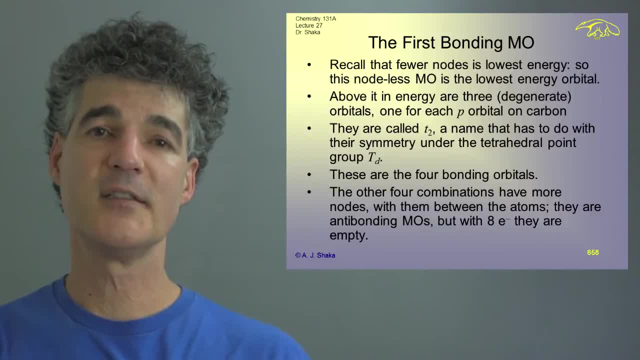 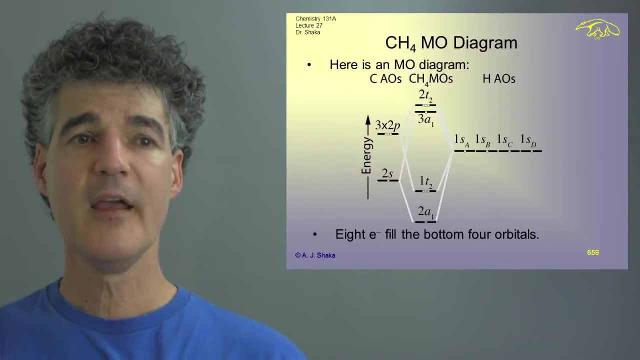 out when you do things correctly, because, not surprisingly, nature finds its way into making the more stable configurations. Here then is an MO diagram. I have 4, it's a little bit harder to draw the tennis tournament when you don't have just 2 players. 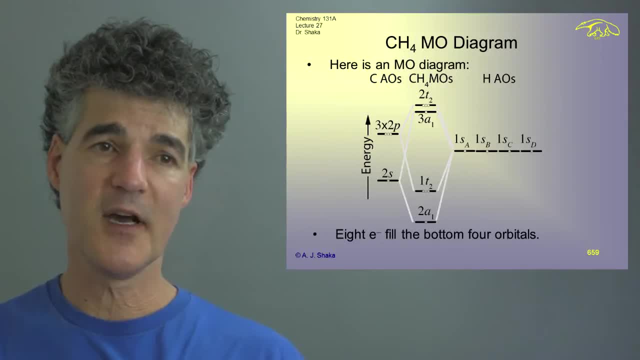 But I have 4 hydrogen 1S orbitals on one side and then I have the carbon orbitals And I have the 2S of the carbon lower than the 1S of the hydrogen. that's good. And then I have the 2P higher. 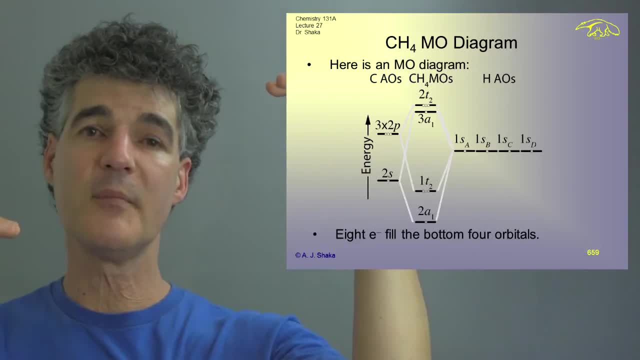 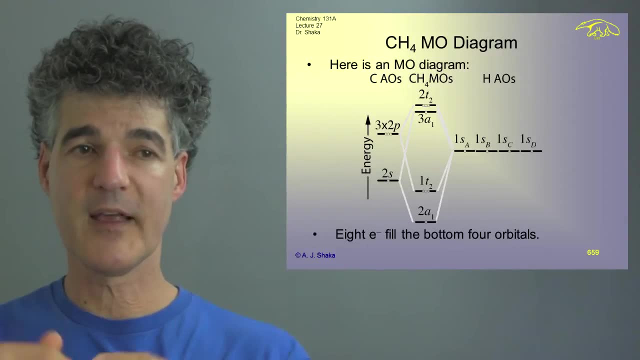 Well, I'd have to know that, but I can certainly figure that out by looking up the ionization energy of the atoms, which is well-known, And so I can order them like that And I have one very good combination: the teddy bear. 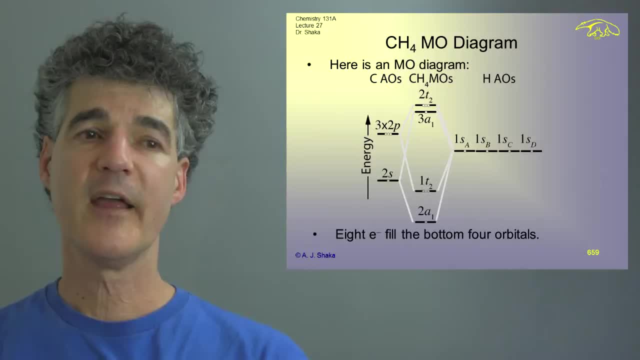 which is down at the bottom, the A1, and then I have the 3 that are identical, the T2. And they're at slightly higher energy. The key is: there's no way that the A1 and the T2 have the same energy. 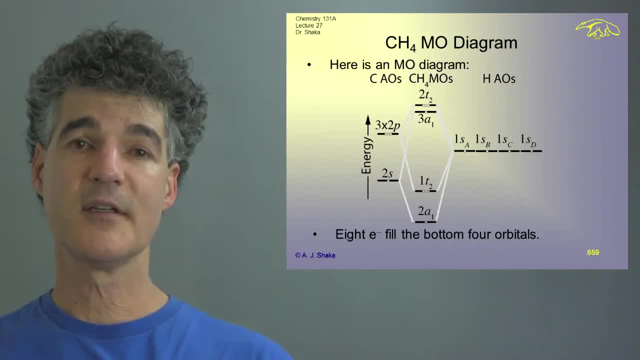 They have to have different energies, And that is an experimentally testable fact that we can look at. So we fill up the bottom with 8 electrons: 4 from the hydrogen, 4 from the carbon, the same way we always do. 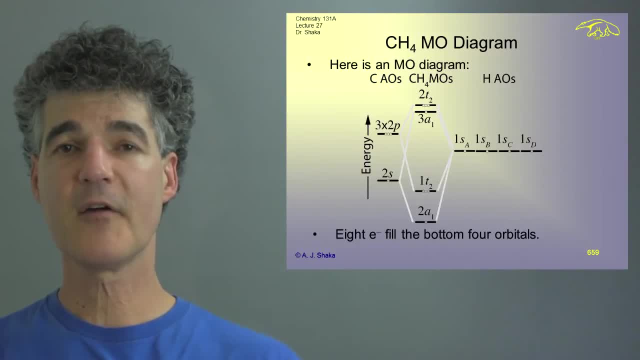 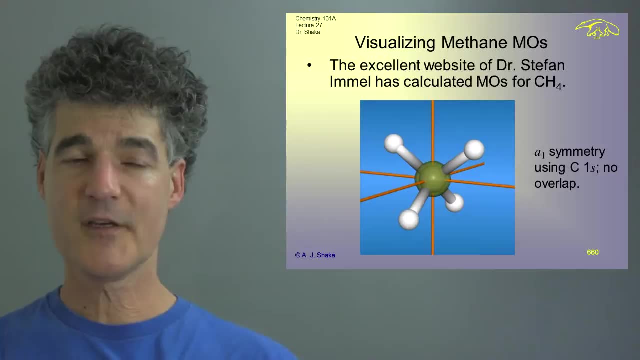 with molecular orbital diagrams. We just once we calculate the diagram, we fill it up from the bottom. And here is an actual calculation of these orbital contours from the excellent website of Dr Stefan Immel. Here is the A1 symmetry between the carbon 1s. 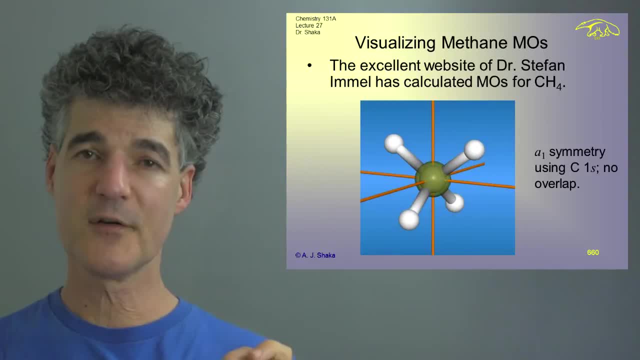 Remember that when we did lithium, when we drew those contours, there was hardly any overlap. What you're seeing here with the carbon 1s is exactly the same thing. The green contour of the carbon 1s is nowhere near the white protons that are sticking out like tinker toy spokes. 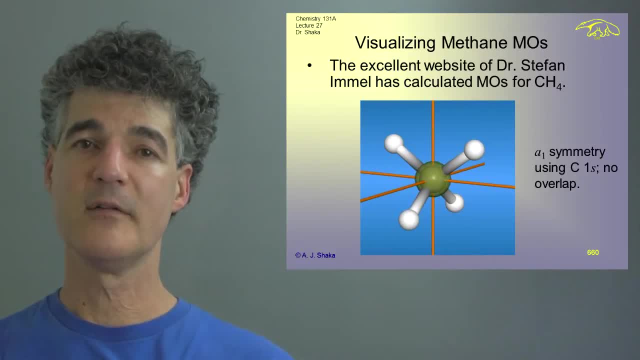 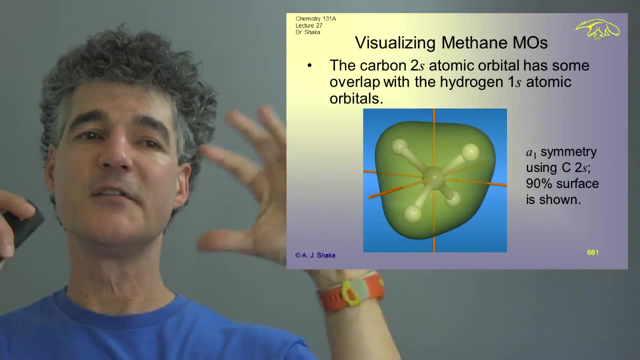 And so the 1s is doing no bonding at all with the hydrogens. On the other hand, when we take the 2s, we get this big spherical look. It can't be exactly spherical because of the underlying tetrahedral shape. 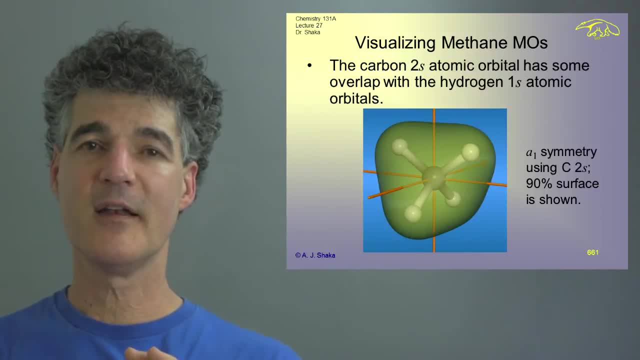 But we get this big green contour And we get this big green contour And we get this big green contour And what's contoured here? the surface is drawn at the 90% probability that an electron in there is inside that region. 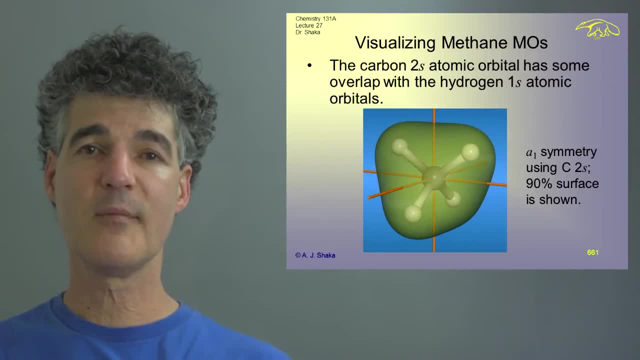 And you can see that it goes around all the nuclei, the carbon and all four hydrogens. So these two electrons in this orbital have this whole big space to go around it And it's a very good overlap with the 1s atomic orbitals of hydrogen. 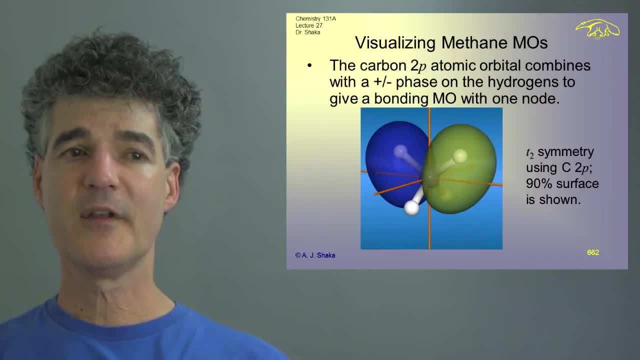 Then the neutrons. The next one up is the 2p And I've shown here one horizontal And the 2p one side is. I apologize, I didn't pick the same colors that Dr Immel picked. 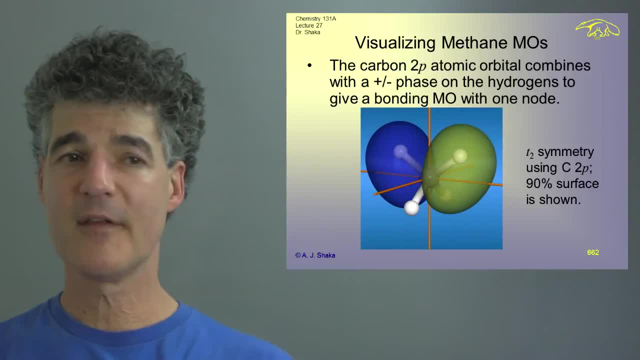 But let's say green is positive and blue is negative, rather than red and blue, same difference. Here there is a node, But the important thing is is that the node is right at the carbon atom. So, although there is a node, 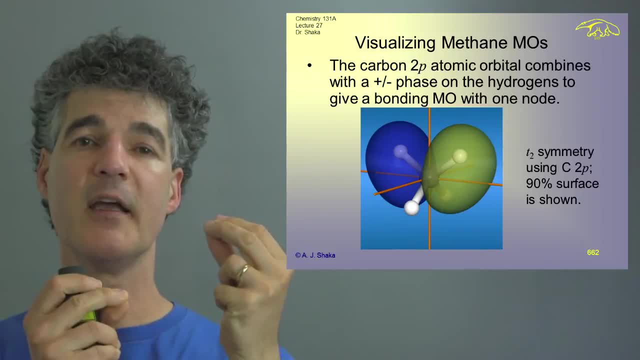 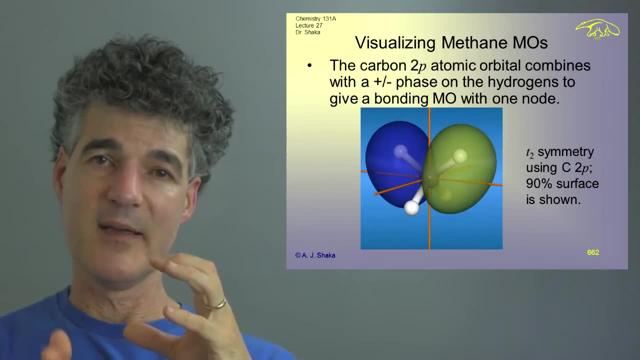 it is not in between the two atomic nuclei. What was bad with H2, with the anti-bonding, is that the node was between them, So that there was no possibility of the electron being in there to glue the positive charges together. 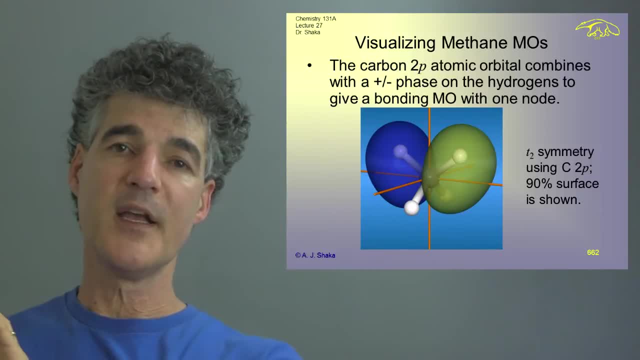 Here we've got one side building up density to hold these two hydrogens in And the other side building up density to hold these two hydrogens in And the node is right at the carbon, where it doesn't do any harm because it's not. 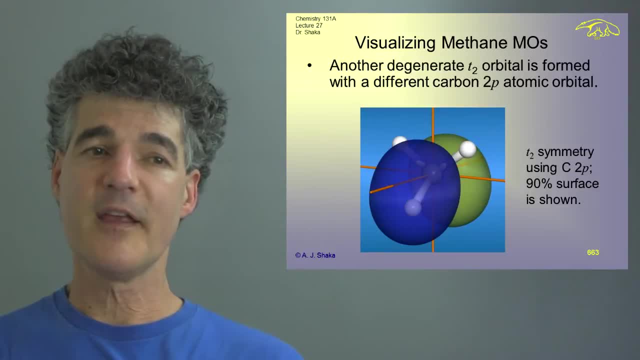 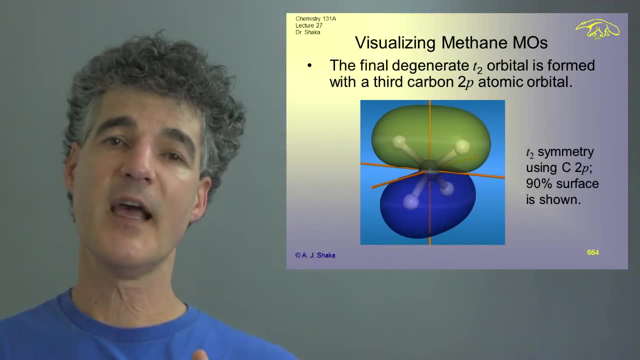 between the bonds. If we look at the other two, they're exactly the same as this one, but they're just flipped. They're all degenerate. They have exactly the same energy because of symmetry. So there's another one that's in and out. 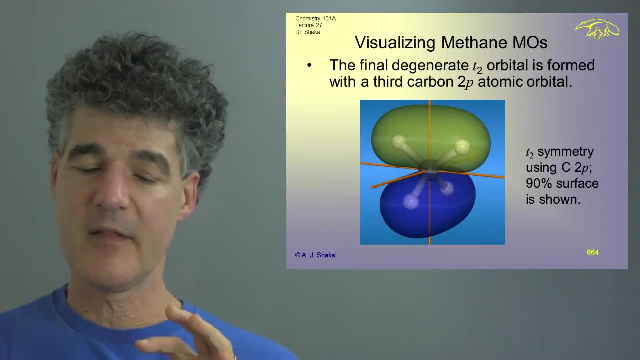 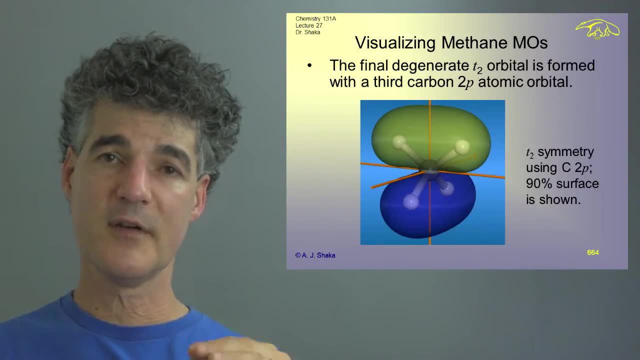 Again, it has a node right at the carbon atom. And then the final one. the third one is just up and down And it's nice. It's nice that he's drawn them with these different perspectives, because as you draw them slightly differently and look, 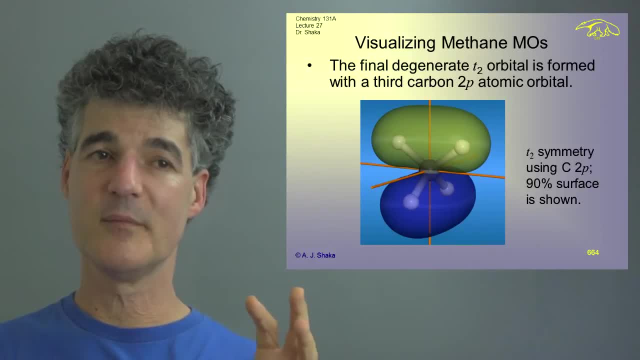 at them, you get a much better idea of what these surfaces actually look like than if you just have one perspective. These are the three then that we said had T2 symmetry, And these are the three other bonding orbitals. They have a node, but it's not a bad one. 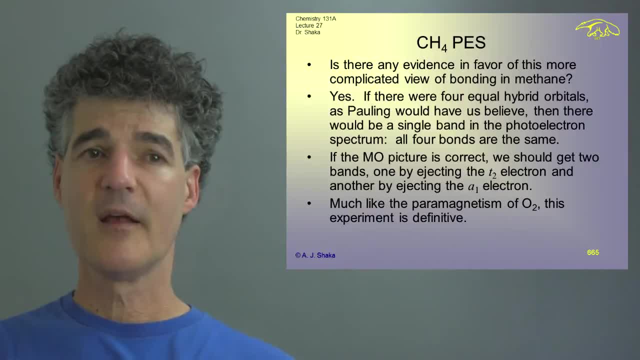 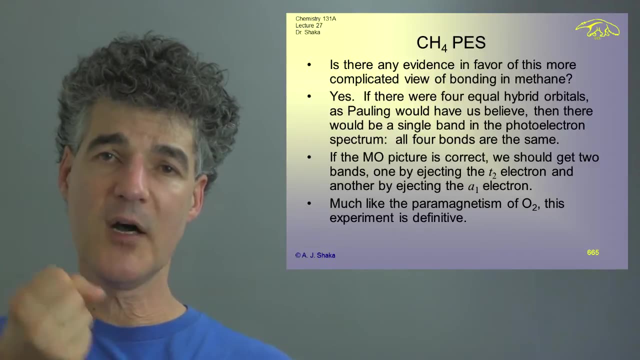 to make an anti-bonding bond. The question is then: on one hand, we have the approach where we first monkey with the carbon orbitals and we keep the hydrogens, And then we make a bond to each hydrogen in turn. 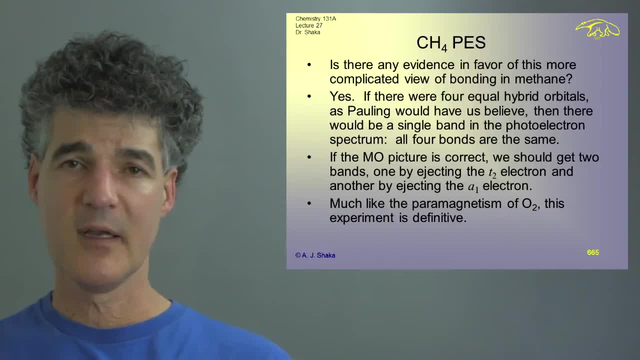 And that's nice because that's how we might draw it on a piece of paper if we were in organic chemistry, for example, or just regular Lewis structure. On the other, we have the MO approach and we can calculate the energy of these orbitals. so I just drew them qualitatively. 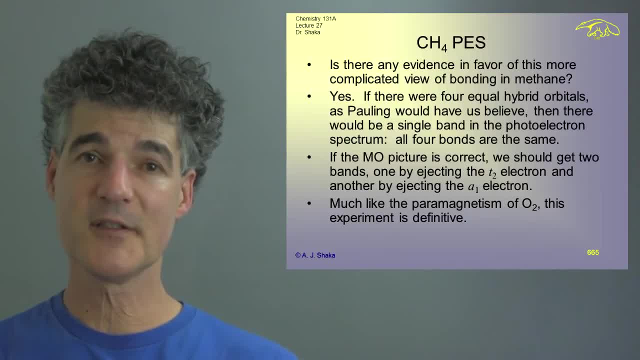 But we can calculate them and under certain approximations, and we can make the approximation better and better if we want to do more work But we don't need to do any more work to say, look in the MO. there are two different kinds of orbitals. 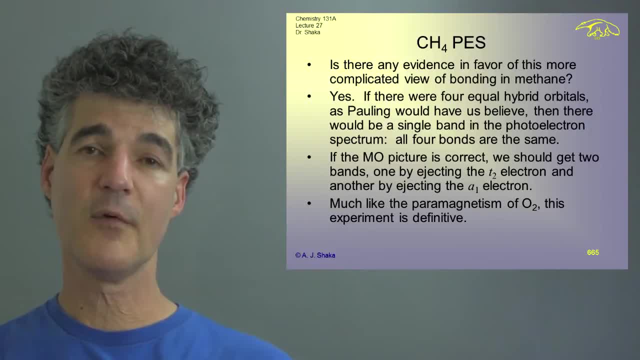 There's one that's T2 and there's a lower one that's A1. And therefore, what we do is we go to somebody who does photoelectron spectroscopy And we say: can you leak in some natural gas and ionize it? 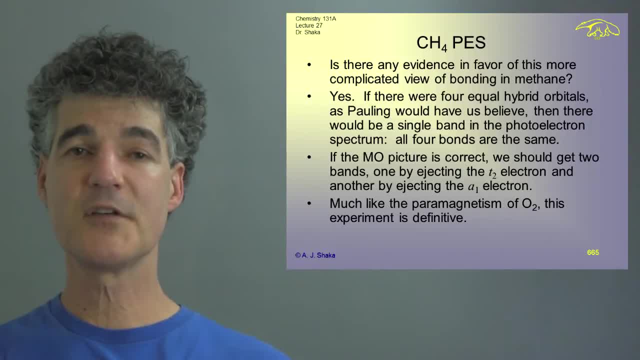 and tell us what the binding energy of the electrons are in this region and how many orbitals there are. And if we do this experiment, there is a difference, because if there are four equivalent hybrid orbitals, each with two electrons, then they're all the same. 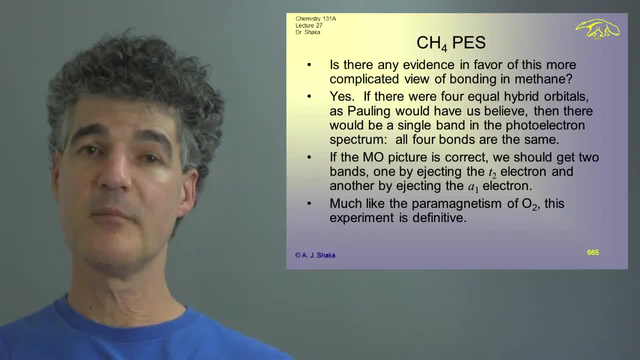 We get one band in the photoelectron spectrum. Pick an electron out of any of those and boom, And you never ionize again. It's so unlikely that you ionize period that you don't ionize twice, So we don't have to worry about that. 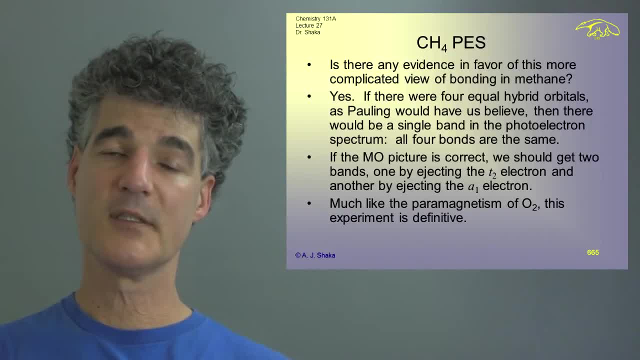 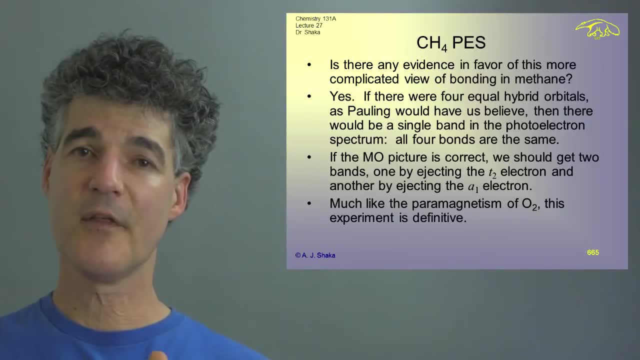 And then the carbon core electrons, which are the only ones left, are much, much higher energy. So we don't have to worry about them either, because we can pick the photon so that they aren't going to come up. We aren't going to put in x-rays, for example. 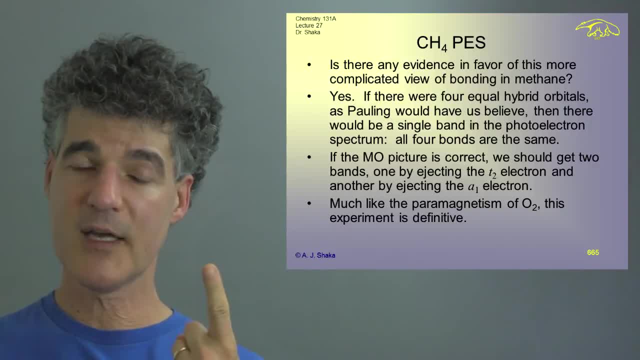 And therefore, if there's one band in the photoelectron spectrum, Pauling is correct And MO theory is washed up. And if there's two bands in the photoelectron spectrum, then MO theory- even though it's a little more complicated and we don't have the stick-like lines- is more correct. 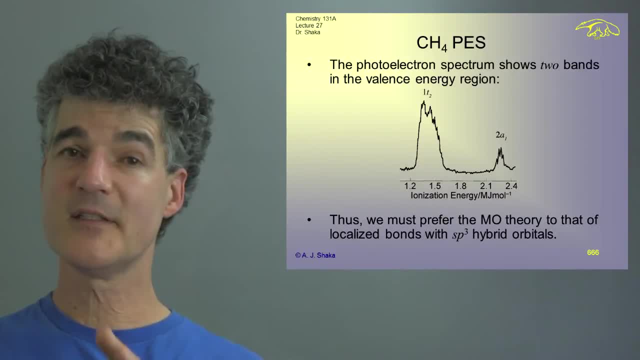 And let's then have a look. And this experiment- just like the paramagnetism of O2, is definitive And of course it comes down in favor of MO theory. Otherwise we wouldn't have gone to all this trouble. Here on slide 666 is the photoelectron spectrum. 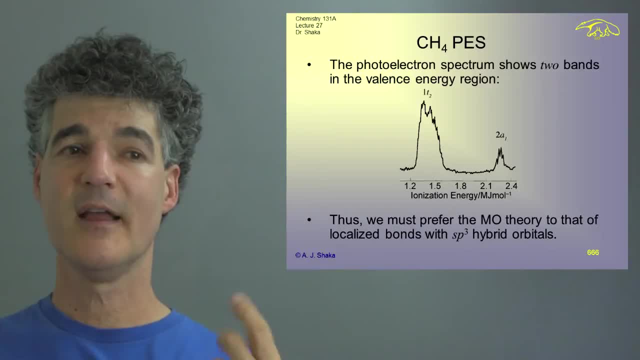 of methane And there are two bands And they're assigned to T2 and A1. And they even have about the right ratio of size. You can see that one looks like it's maybe three times bigger than the other. There are a lot of factors that go into the cross sections. 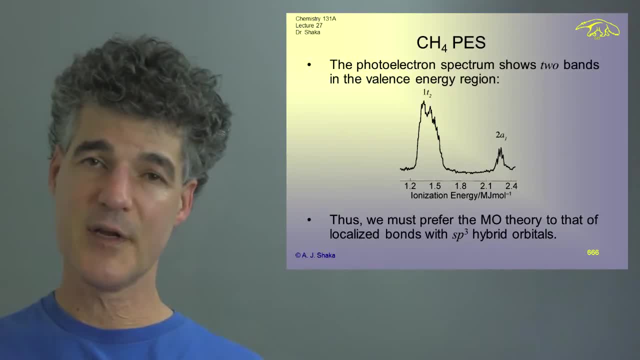 of photo ejection. So you can't just say if there's three orbitals you get three times the area, or anything as simple as that. But nevertheless it does seem to make some sense. And if we look at it, the vibrational progression. 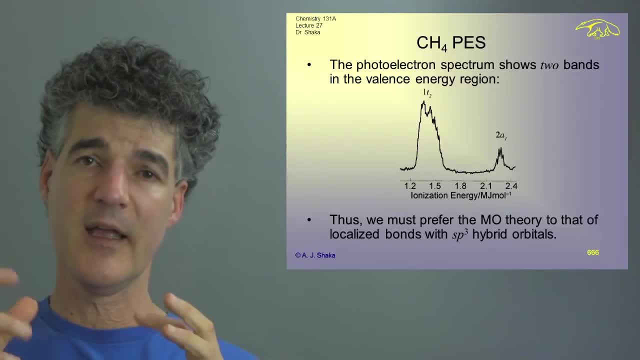 because methane is a much more complex molecule and can really vibrate in a lot of different ways, Which is, of course, one reason why it's a very bad greenhouse gas, because you put it up in the atmosphere and it can absorb infrared in a lot of different ways. 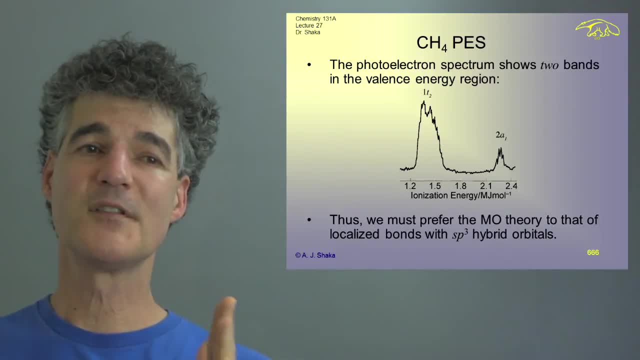 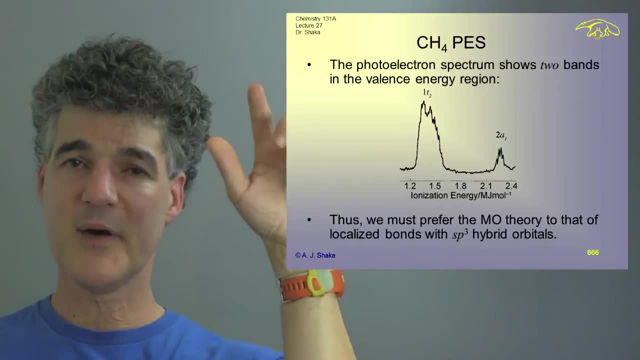 and then radiate it back down to Earth. We can't resolve all the little things like we could in N2. They just appear as kind of a ragged, like a porcupine envelope, But nevertheless we can say it's the T2 really that's doing. 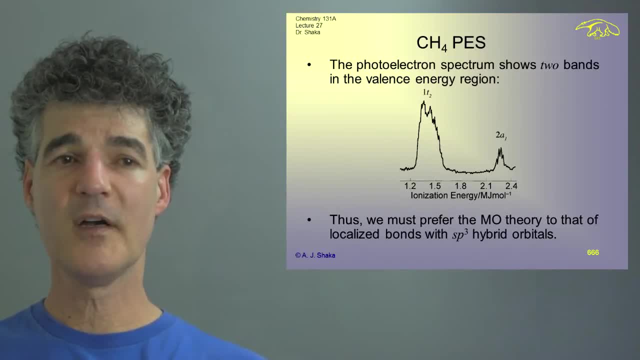 the lion's share of the bonding In methane and the A1, the big teddy bear is rather less important because of the less vibrational progression when we eject an electron from it. This then says: look, we have to prefer the MO theory. 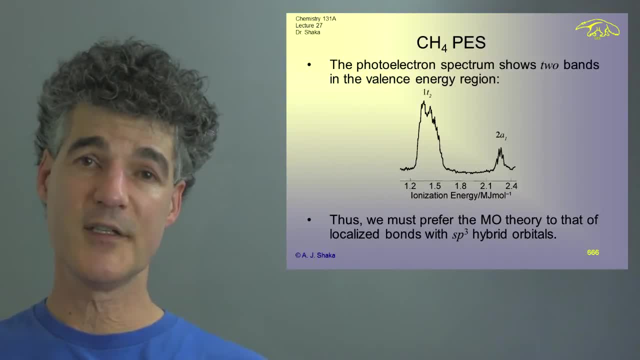 to the theory of localized bonds, even clever localized bonds with hybrid orbitals, because now we have an experiment that's clearly indicating that one approach is better And it disagrees with the other one. And that's what science is all about. It's easy to talk, but you can talk all you want. 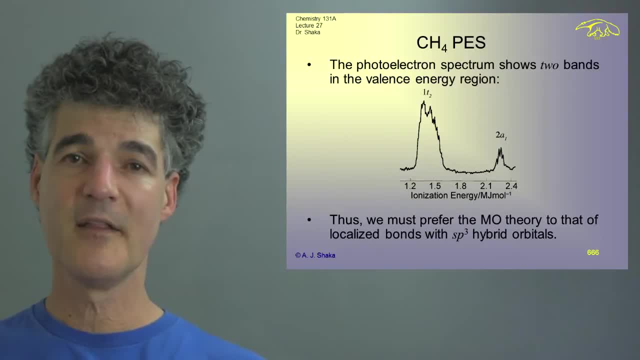 If somebody does an experiment and shows the ocean is rising, then it's rising And it doesn't matter whether you want to say it's not or if it's measured. you can quibble with the measurement, But you first have to understand how the measurement works. 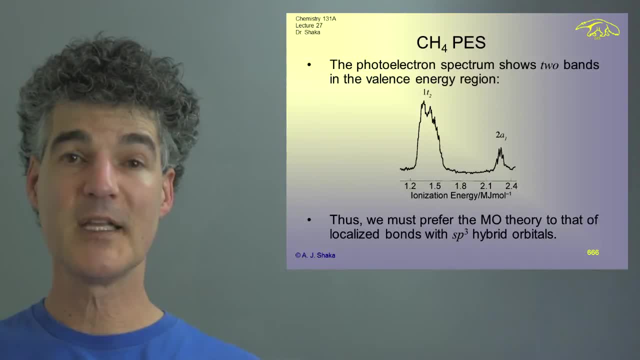 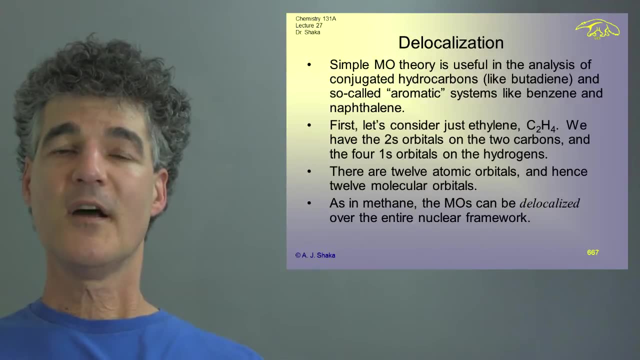 And in fact the measurements along those lines are extremely reliable, even though the system itself is quite complex. So we can't say it's not, It's complicated. All right, let's talk about some bigger molecules. We don't want to just leave off with methane. 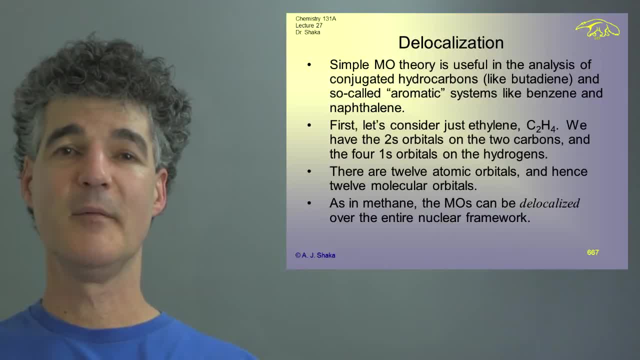 Although to a physical chemist, methane is a big molecule in a lot of ways, And I think you can see why: because they may want to know a lot of things about it that an organic chemist may not be interested in and an engineer just wants. 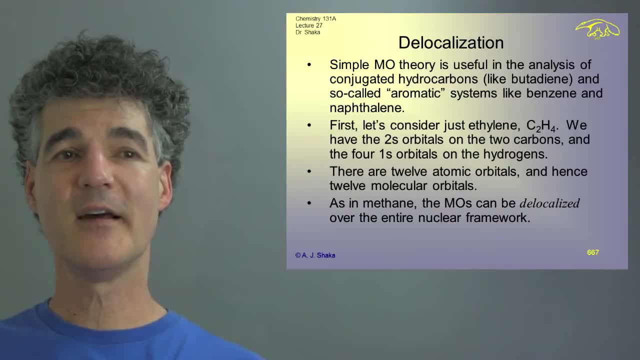 to burn it and get some power. So we can look at some of these, Some conjugated hydrocarbons and so-called aromatic systems. I've never smelled an aromatic molecule that was aromatic to me like a rose, but they're called aromatic. And they certainly do have smells, but they usually smell like gas or mothballs or something like that. But let's look at benzene, naphthalene and a few others butadiene, so-called conjugated Hydrocarbons. 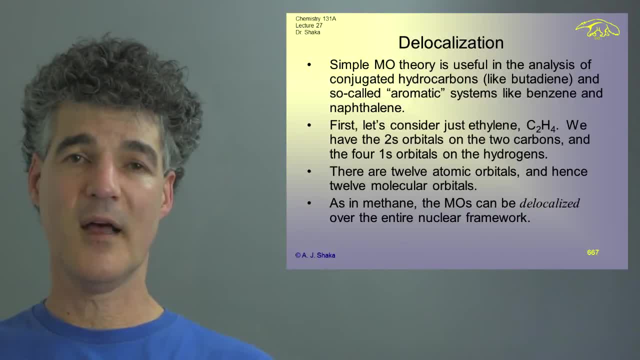 And this will be kind of an interesting- another interesting way to simplify what could be an extremely complex- if we did it from scratch, it would just be terrible calculation- and make it simple and leave enough meat on the bone that we can still come. 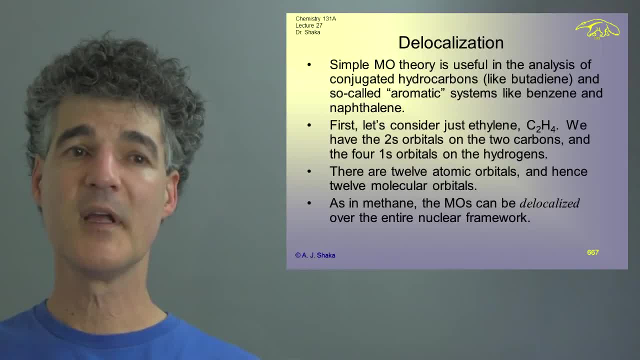 to some interesting conclusions about the stability of the system. First, let's just consider ethylene C2H4.. Ethylene is an extremely important molecule in the fine chemical industry. It's the feedstock for a lot of things, And a lot of people are spending time and energy to figure out how. 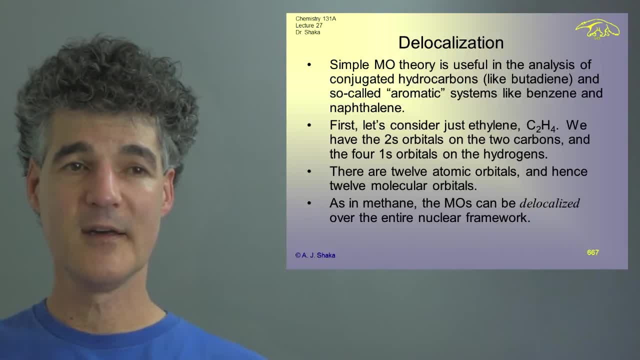 to make ethylene efficiently when we run out of other ways that we have been making it. Well, we've got the 2S orbitals on the two carbons and the 2P orbitals and we've got the four 1S orbitals. 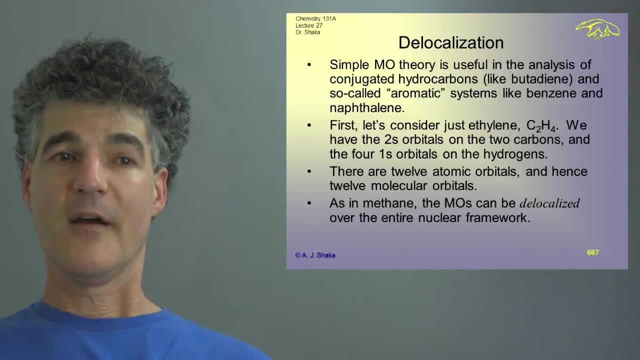 on the hydrogen. So there are going to be 12 molecular orbitals and because there's 12 atomic orbitals- and 12 is a lot, but we can still figure out what they should look like. Just like methane, even though this is bigger. 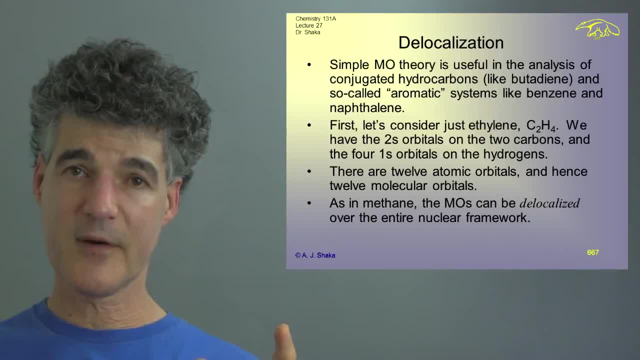 we're going to have to start by putting the nuclei at their preferred position- 120 degree bondage, bond angles between the hydrogen and the carbon, And then we're going to have to solve for what the molecular orbital energy should be by putting in electrons that are allowed to go. 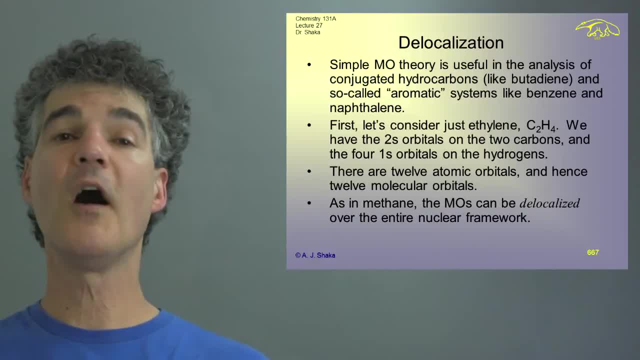 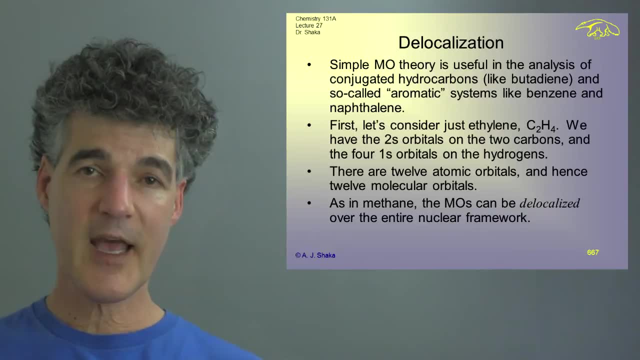 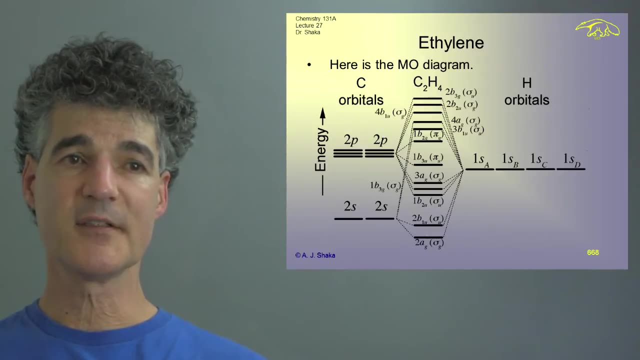 over the entire nuclear framework, And only if they don't want to go over here for their own reasons are they not going to. It's not that we're capturing them between two nuclei Here then on. 668 is the hydrogen. 668 is the molecular orbital diagram for ethylene. 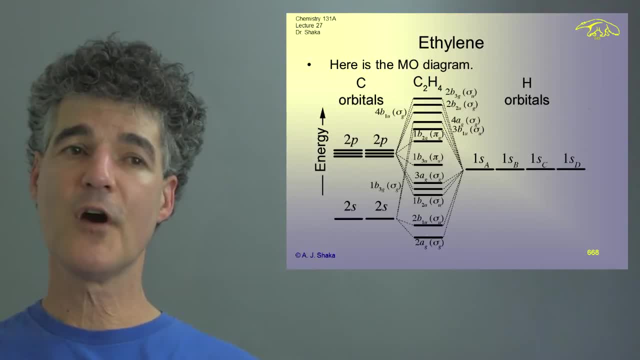 We've got our four hydrogens again, but now we've got two carbons And we've got all these states labeled from the bottom sigma G, 2AG, with symmetry labels 2B, 1U, and so forth and so on. 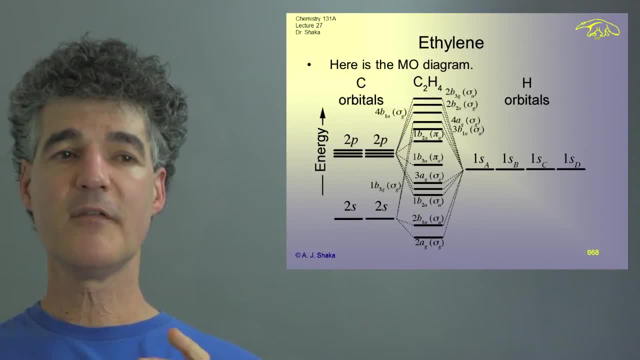 We don't have to understand what all of them mean, but many of them are overlapped between the S orbitals on carbon And the S orbitals on the protons. And then there's two right in the middle there, marked pi G and pi U, that are just coming from the carbon. 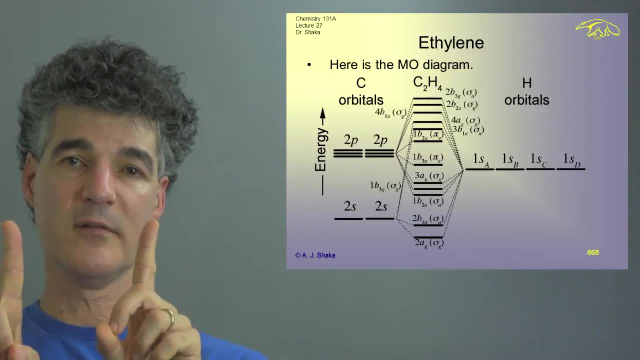 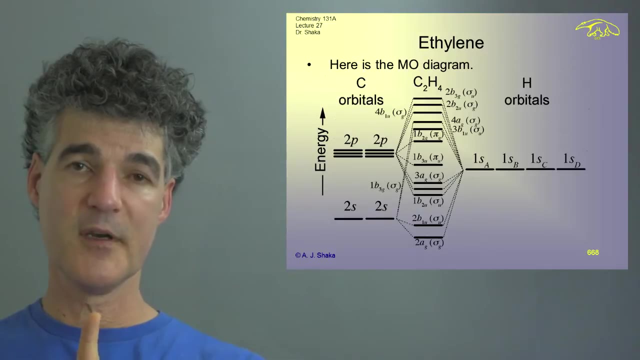 And that's because those two are orthogonal to the plane in which the protons are. So those two have different symmetry than what the S can be And therefore they only come from the carbon. They can either be this way, the two carbons, or that way. 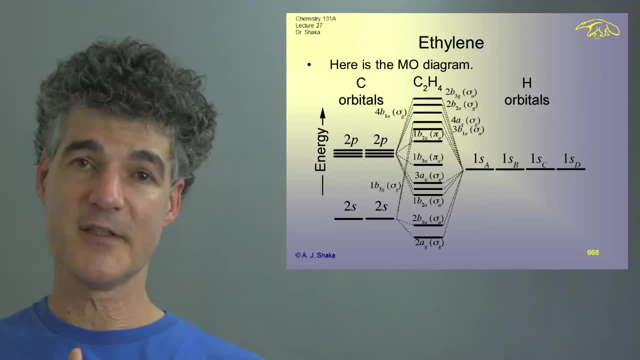 And of course only one of them is filled, because there's one double bond in ethylene: There's a sigma bond and then there's a pi bond, And so one of those is filled right up to where it's stable. They're slightly below the 2P level. 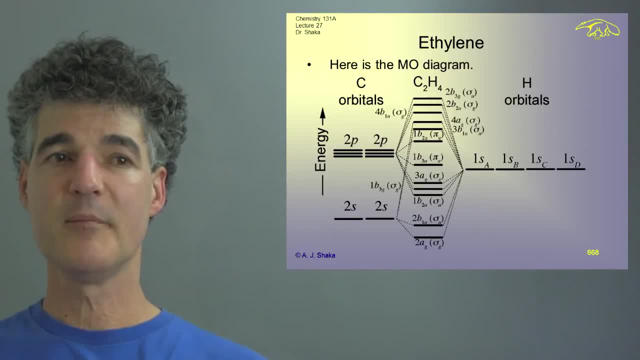 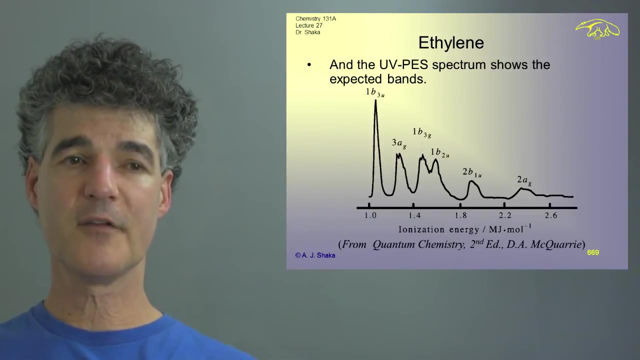 We slot in all our electrons all the way up. What we find is that it's filled in the two pi bonds, That it's filled right up to that level. that involves just the pi orbitals of carbon, And here is the photoelectron spectrum of ethylene. 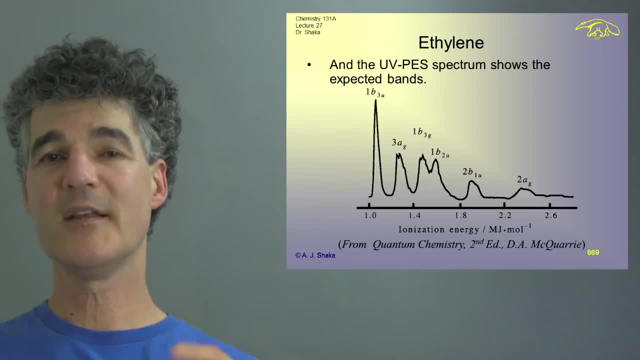 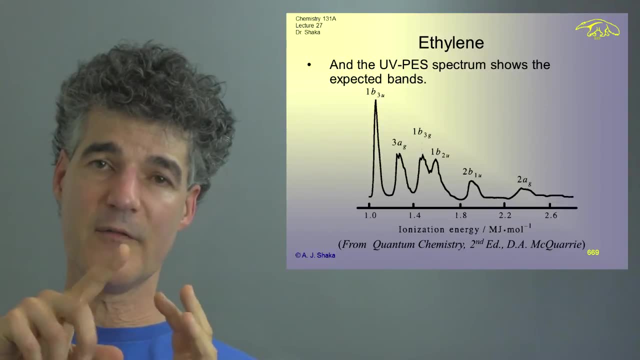 We can also get that. And now the ethylene is quite complicated. So these peaks that all have vibrational progressions are very, very hard to resolve And they end up they may not be resolvable at all. It depends how. 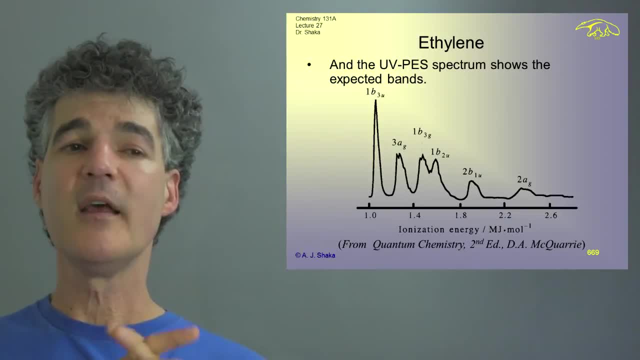 It depends how carefully and how clever the experimenter is, But at least they aren't so wide that they overlap with each other and we can't see them at all. And they've all been assigned as you can see: 3B3U and 3AG. 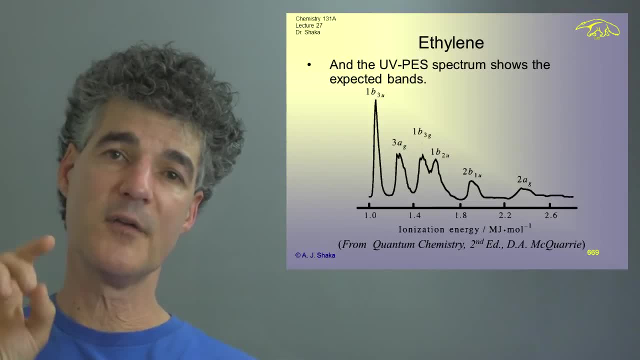 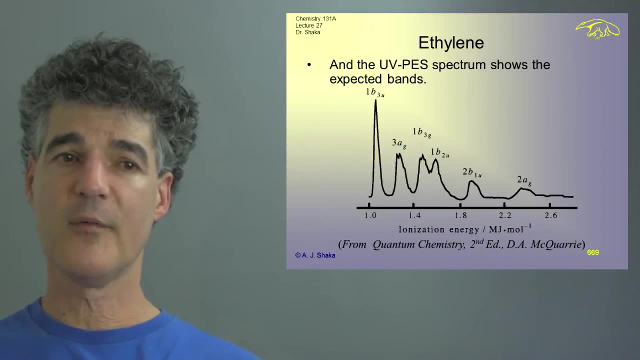 and so forth, and they're all assigned And they all correspond to ejecting electrons from lower and lower in the molecular orbital diagram all the way to 2AG. after that, Maybe you need two more, Maybe you need three more, Maybe you need three more. 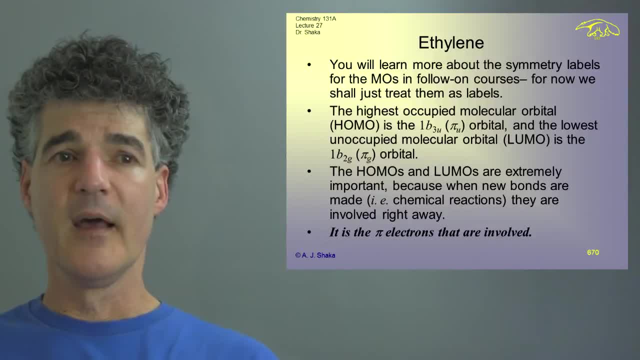 But they all have pretty much energy and they didn't have such energetic photons. The symmetry labels again. treat them just as labels. for now Don't dwell on them too much. Once you study group theory, you'll know exactly what they mean. 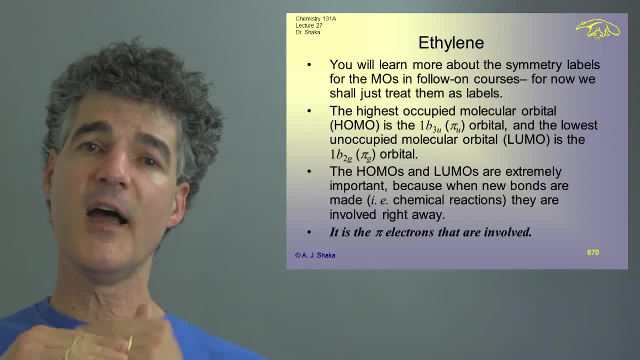 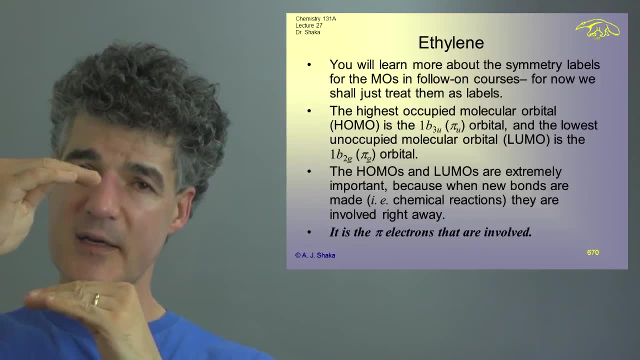 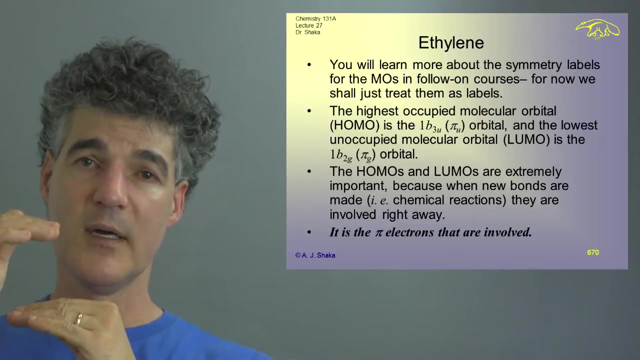 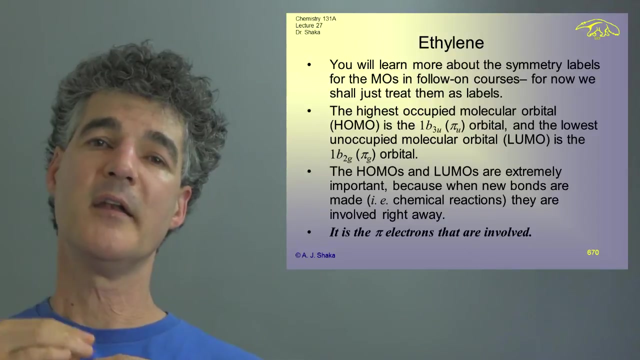 For us, though, it's the highest occupied molecular orbital, the so-called HOMO, and the lowest occupied- excuse me, the lowest unoccupied molecular orbital, the LUMO, that are going to be the most important thing. Why? Because, if I'm going to be making a bond, 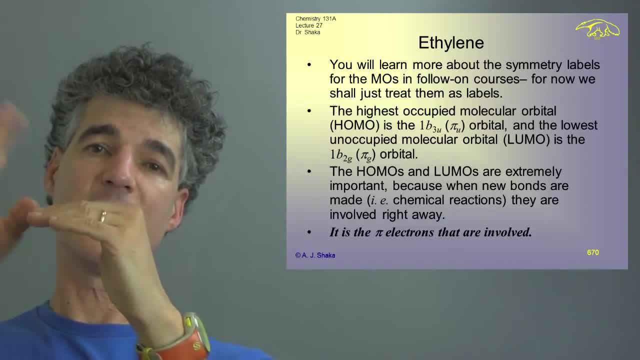 then it's the electrons right at the top of the cake that are going to fly off and go somewhere and make the bond. The ones that are held down further down in energy are not going to be likely to be the ones going first. 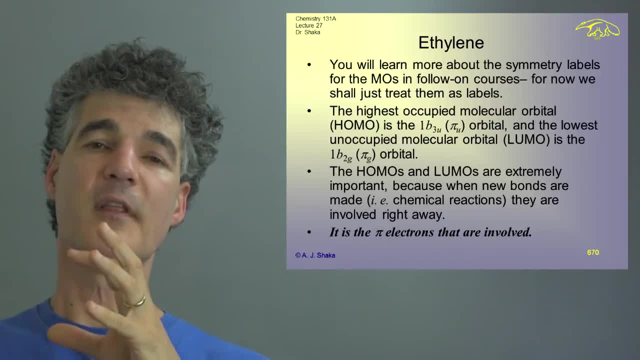 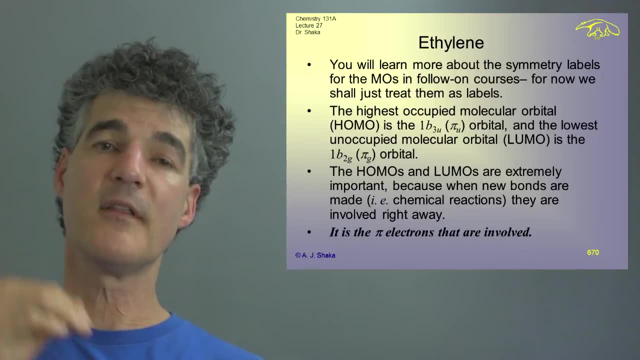 And likewise, if someone is going to be going first, then some other atom is coming up brimming with electrons and says: hey, take some electrons from me. Where are they going to go? Well, they're going to go into the lowest unoccupied molecular orbital. 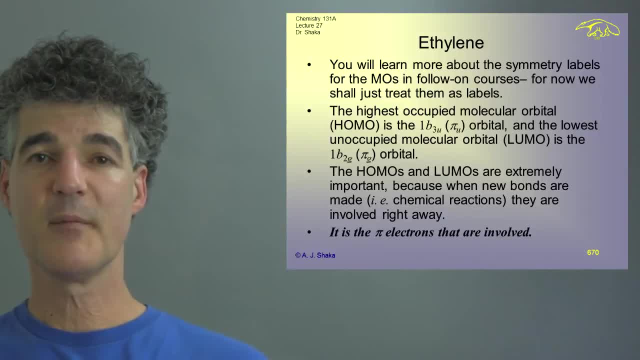 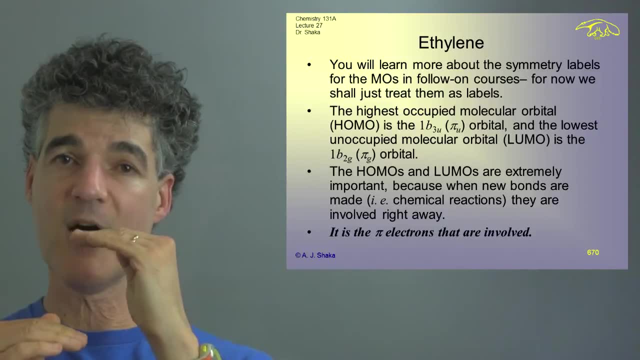 because they're going to come in and they're going to go down to the most stable state And therefore the highest occupied molecular orbital- what it is- and the lowest unoccupied molecular orbital- what it looks like- are very, very, very important. 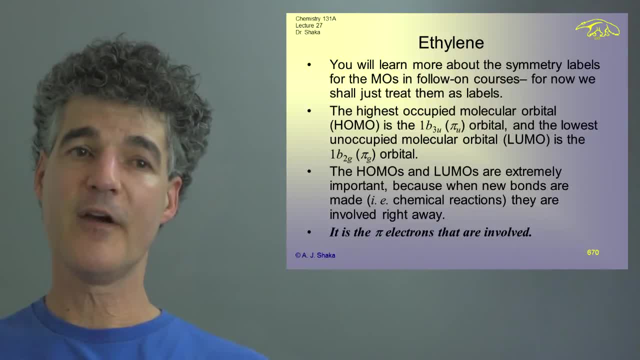 to understanding, And that's what we're going to talk about in the next class. And that's what we're going to talk about in the next class. So let's talk about the most unoccupied chemical reactions And therefore we can focus mostly on them and forget. 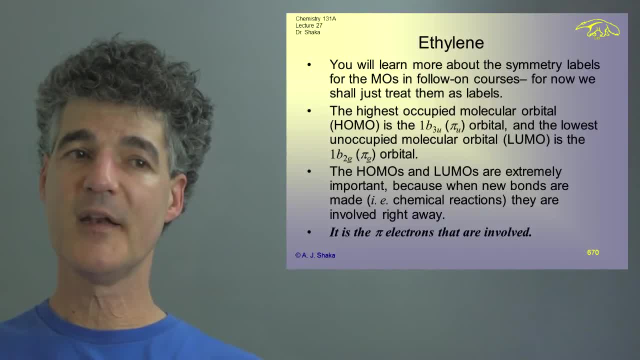 about most of the other ones, And that's a key simplification. The highest occupied one I've labeled as 1B3U and the lowest unoccupied is 1B2G, And they both involve the carbon P, which is the highest unoccupied molecular orbital. 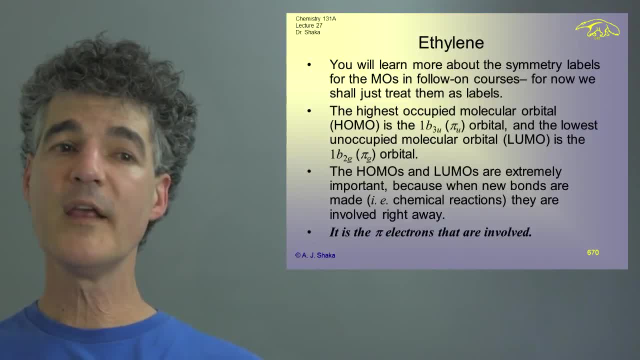 And so these two, the highest occupied and the lowest unoccupied, only involve pi electrons. It's only the pi electrons that are involved, And that is a key simplification when you consider the reactivity and structure of things with double bonds like ethylene. 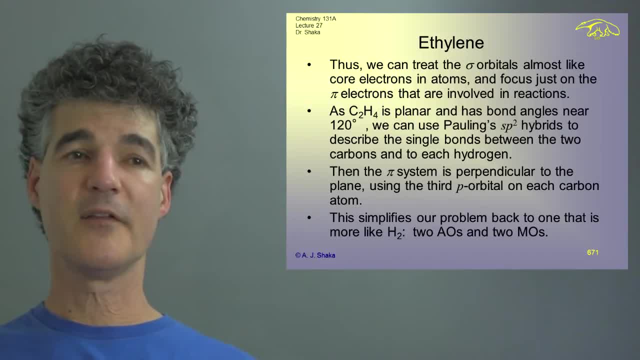 We can treat all the sigma orbitals as just like core electrons, And since they aren't important, they aren't going to be participating. we can rationalize whatever structure they have in any way we want, And usually the prescription is: those aren't so important. 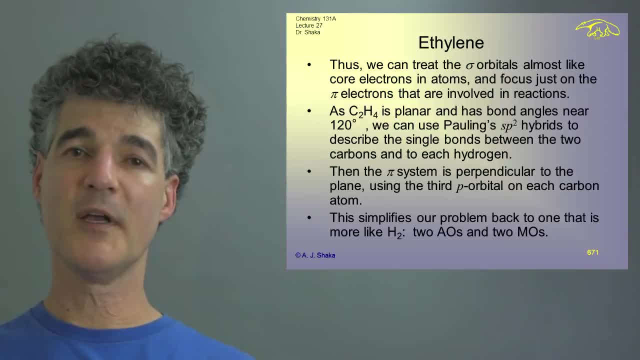 we just say they're SP2 hybrids. It doesn't matter what we call them, because they're never going to do anything, They're just going to be filled. And we might as well take a simple approach, like Pauling's approach, and just say: well. 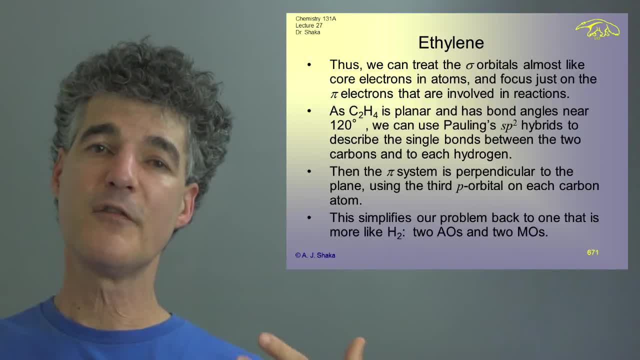 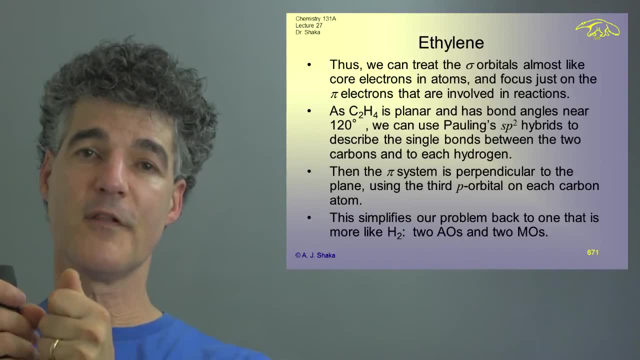 they're making 120 degree and that there's a sigma framework that's holding the atoms in place. And then there's these delicate pi orbitals, And for those we reserve the molecular orbital treatment, because those are going to do something, And so we want to treat them more accurately. 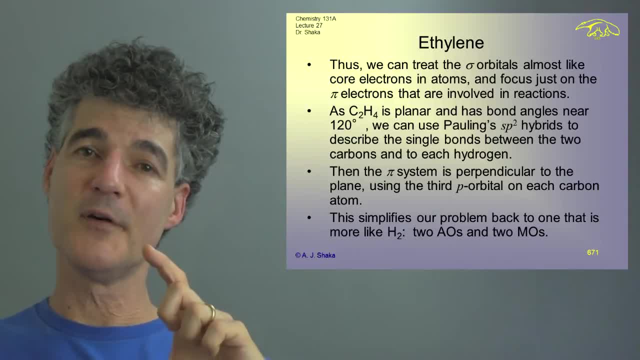 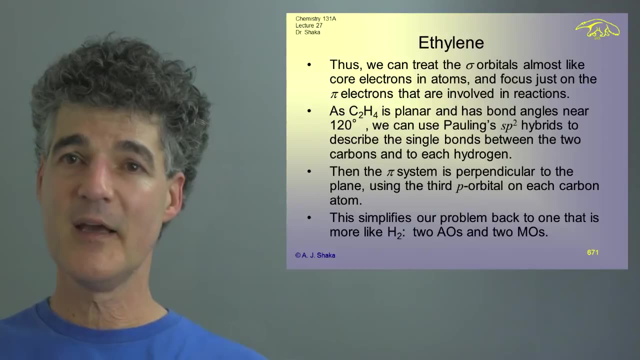 And because there's only two orbitals, this and like that, it's basically down to the same thing as back to H2.. The fact that they're P right Rather than S doesn't matter. The math is exactly the same and we've already done it. 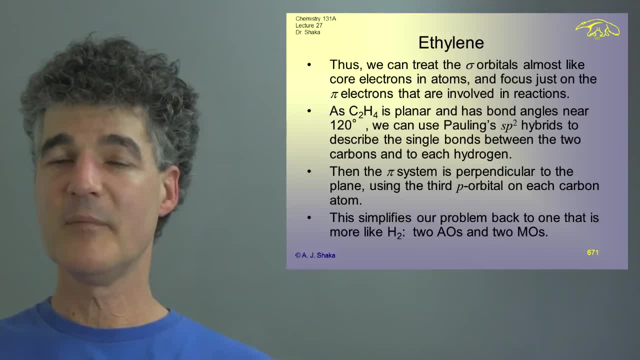 So we can leverage that now and just say we've got this perpendicular pi system with two P orbitals and they can either be in phase or out of phase and we can calculate what we want to do. So it's just like H2 in this case. 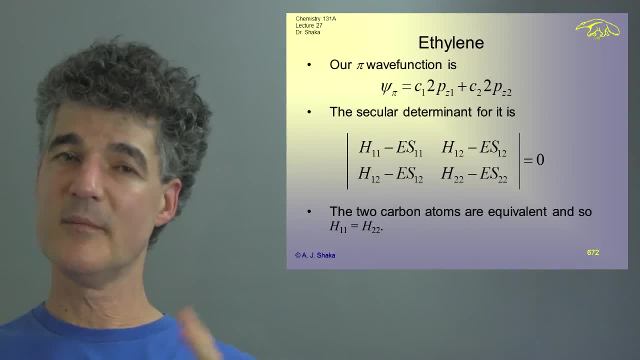 Our pi wave function, then, while we suppose the molecular orbital for the pi Is C1, 2PZ1 plus C2- 2PZ2, where 1 and 2 are referring to the two carbons and C1 and C2 are the two coefficients, 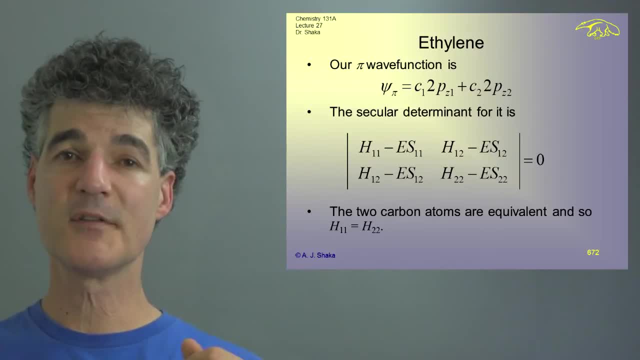 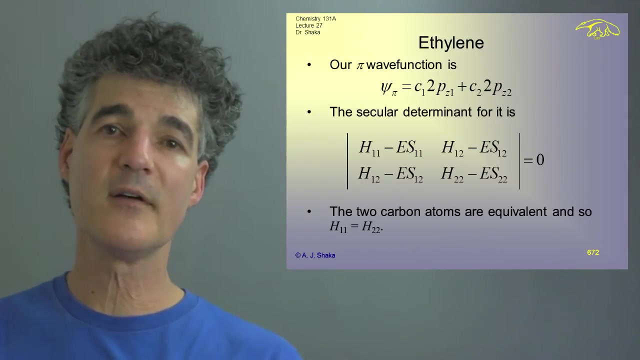 yet to be determined, but we know they're going to come out to be equal because the carbons are the same by symmetry. We have to make a secular determinant because this is molecular orbital. We've got to calculate the orbital Energy is. remember we have the Coulomb integral. 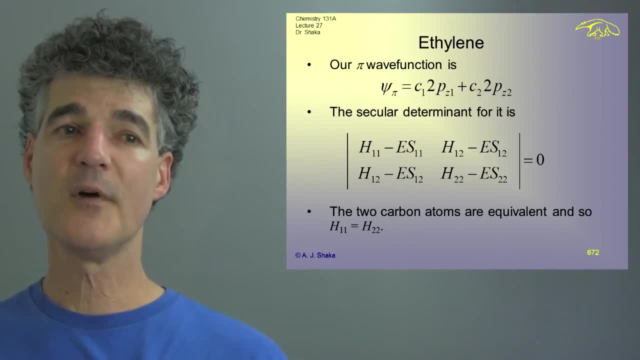 and the exchange integral, and so here it is H11 minus ES11, we have the overlap integral, H12 minus ES12, we have the exchange integral, and so forth. The determinant: so this times this is equal to zero. and since the two carbon atoms are equivalent, then H11,. 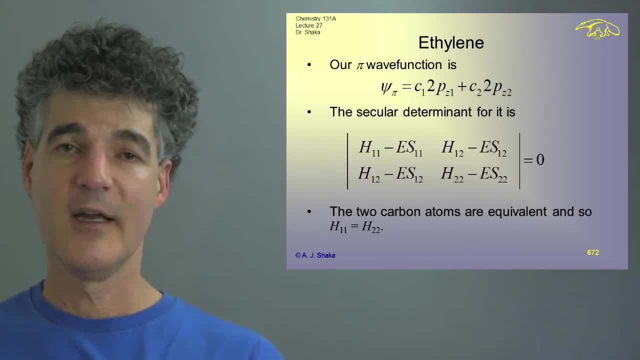 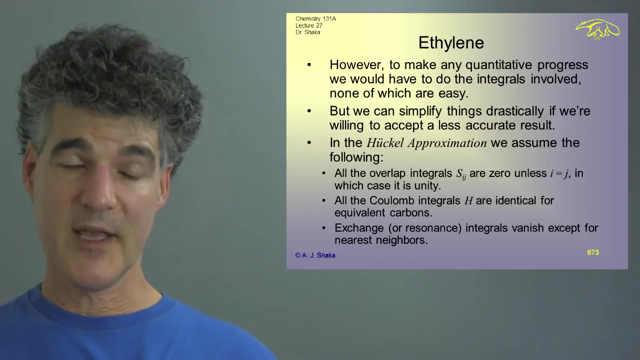 that integral And H2. And H3. And H4. And H2, that integral are exactly the same, so we can make those the same and H12 is already the same. So if we wanted to make quantitative progress here and we wanted to proceed the way we have in a lot, 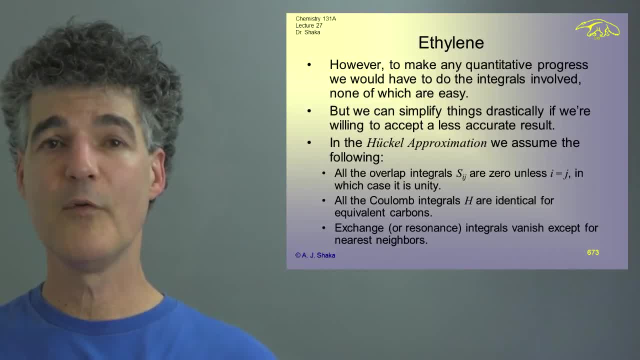 of other cases- helium and hydride- we'd have to get out our integrals, our thetas and sine thetas and all that and go to work. but we don't want to do that. None of that, None of that's too easy to do and we're only 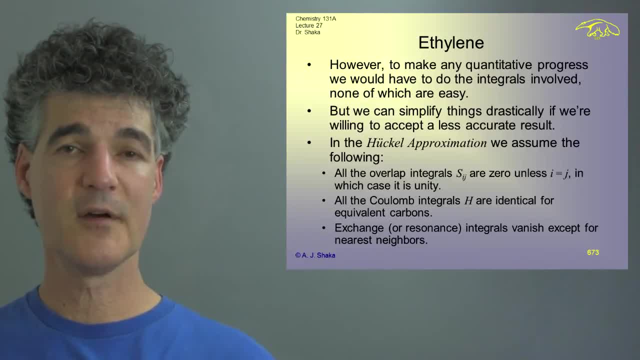 after some qualitative description of what's going on. We don't expect it to be quantitative. It'd be very hard to make it quantitative, even if we calculate these pi orbitals so well, by just leaving out everything else and saying: forget it about the other stuff. 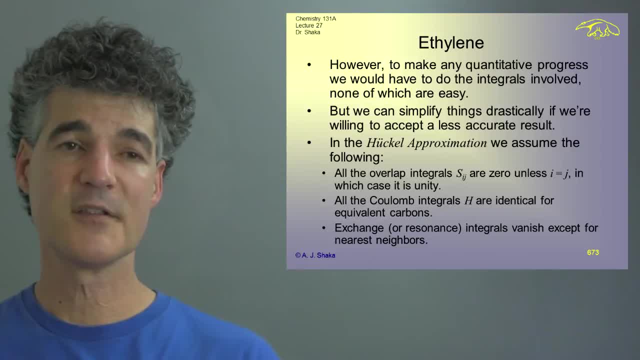 We could be making some big mistakes, some big errors there. Let's simplify things and not do any any integrals at all, and that will be a very, very good method, and that's called the Huckel approximation. An integral, whatever it is, is just a number. 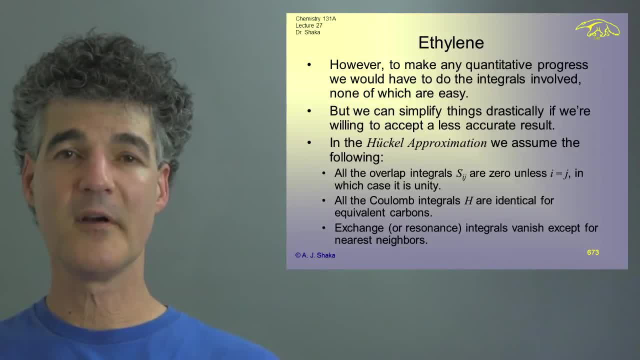 by the time you integrate it, It's a number with units, but it's a number, and we're going to assume that we're going to just replace integrals with these symbols- numbers, alpha and beta- and we're going to calculate things very quickly then. 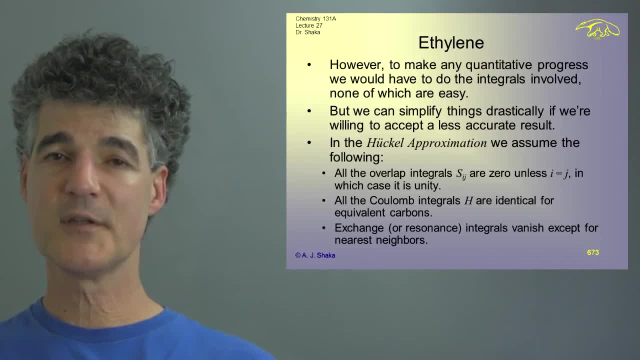 The Huckel approximation makes three assumptions And at first they seem laughable, but in fact they're very nicely physically motivated. The first thing is the overlap integral. Remember how much trouble that was to calculate S and how we had to do all those things. 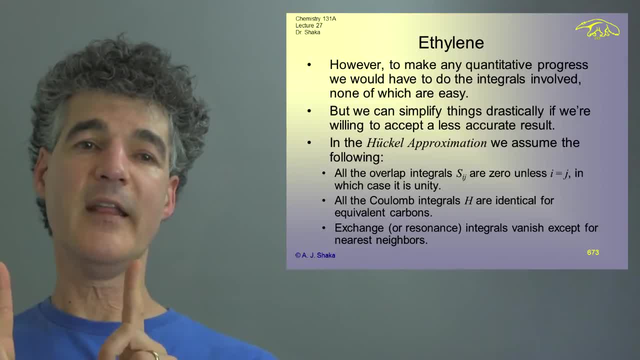 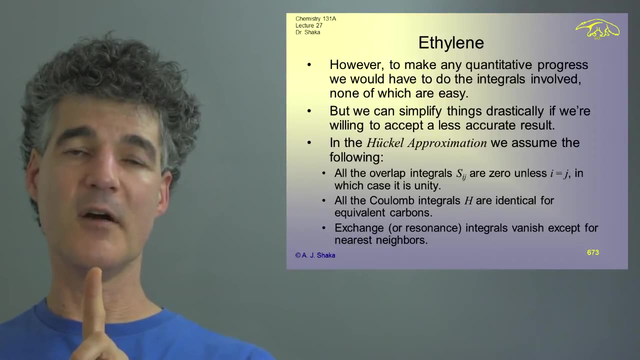 Well, here, what we're going to say is this: We're going to say that the overlap integral is zero, unless you're talking about the overlap to the same place. So the overlap even between two neighbors is zero. Now that seems very counterintuitive. 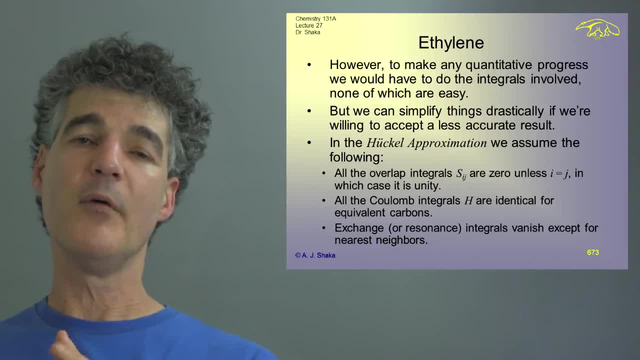 Why? Because you're claiming they're making a bond, But when you look at what came out of our analysis before, S was just a player in the denominator. that just changed things slightly in the denominator. It never dictated whether a bond formed or not. 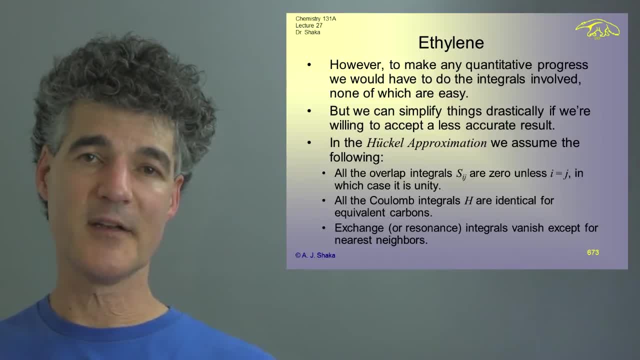 It was OK. so it doesn't really matter if we set it to zero. And if we set it to zero, then we're getting rid of a lot of math because all those things go away, because they're multiplied by S12.. So those are gone. 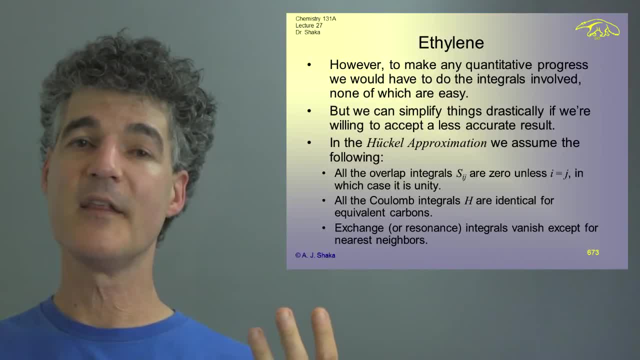 And then when it's the same, we set it to one because we're saying it's normalized. And then all the Coulomb integrals, the H integrals, are the same for equivalent carbons And sometimes we assume they're the same even. 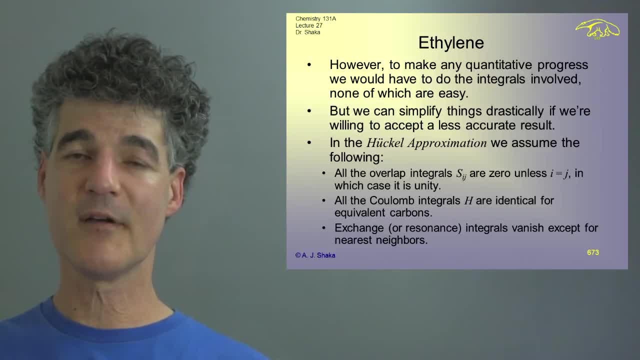 if the carbons aren't quite equivalent, because we're just too lazy to figure out if they're that much different, or we, or it's difficult to figure out what they would be. And then the exchange, or they're also called resonance integrals. in the business, those integrals vanish, except 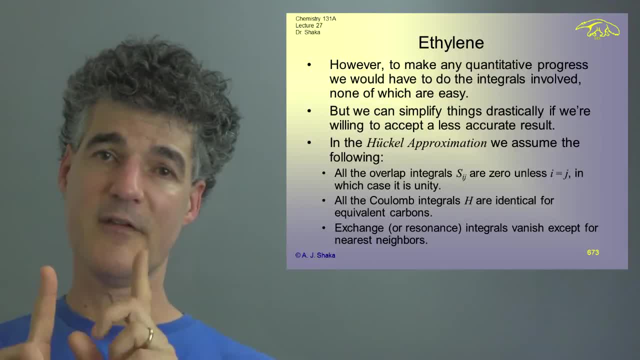 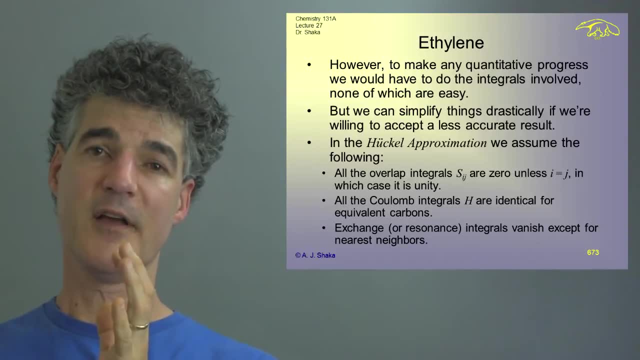 for nearest neighbors, And the rationale for that is that if I'm here and you've got a P orbital, then that integral is going to have some value. But once I get out to here and I've got something intervening in between, it's too far away. 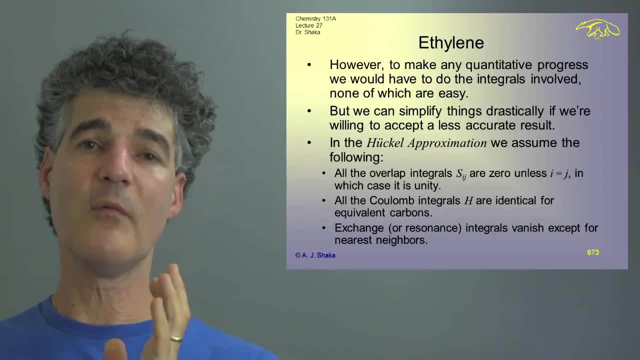 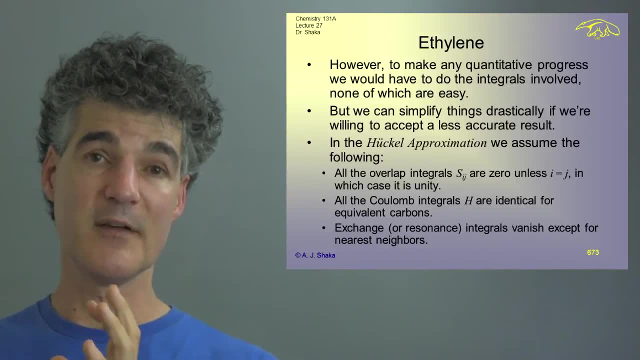 So I could calculate it, but it'd be small And I don't want to waste all my time calculating something that is 0.1% of the answer but is extremely difficult to calculate. That's a poor use of my time. 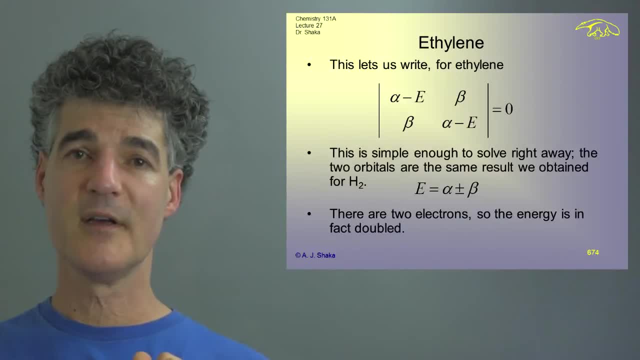 So those three approximations. let us simplify our secular determinant and get rid of all the calculations. Conventionally you write alpha for the P orbital, So that's 0.1%. We're one of the integrals in beta for the exchange. 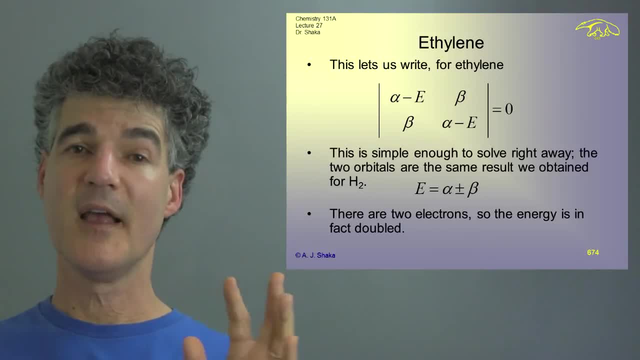 And our secular determinant just becomes alpha minus E, beta, beta. alpha minus E equals to 0. And if I that's a quadratic equation and the solution for the energies is alpha plus or minus beta, Not surprisingly, it's very similar to what we had with H2.. 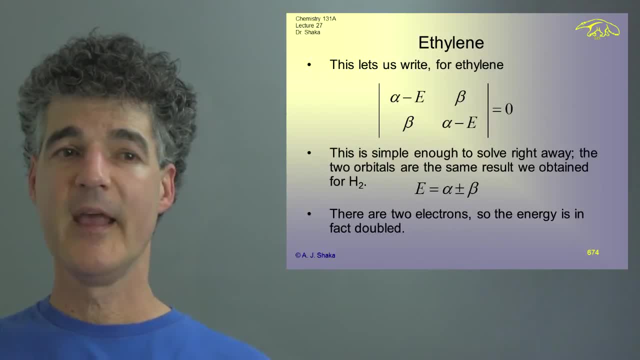 There's a good combination And a bad combination. Now, in fact, there's two electrons going in, and we didn't calculate any electron-electron repulsion or anything like that, So all we're going to do is double the energy when we say what it actually is. 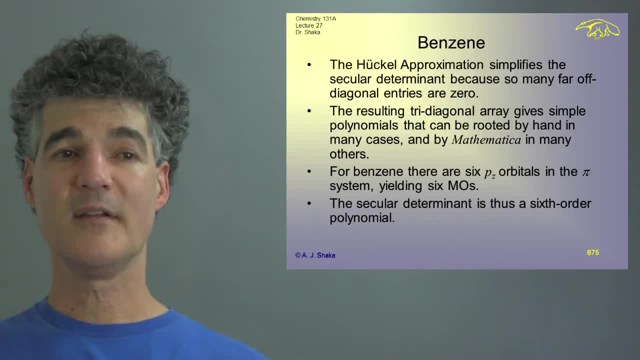 The advantage of this, however, is we can do something that's a little bit more intimidating, much more intimidating than helium, for example. Let's try benzene: Benzene, It's C6H6.. We would have a 6 by 6 determinant. 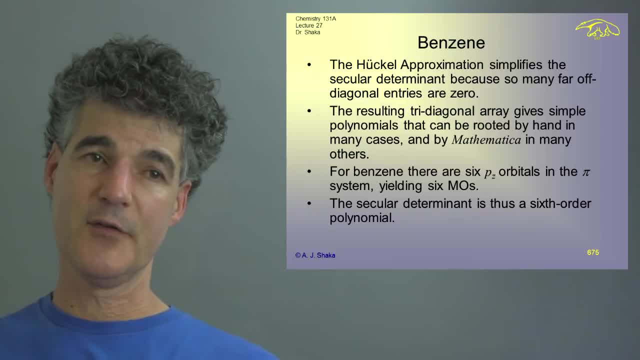 and it would have entries everywhere. So just expanding that out as this times the determinant of the 5 by 5 plus this will take forever And that's going to be a major problem to try to calculate something like that. So let's figure out how. 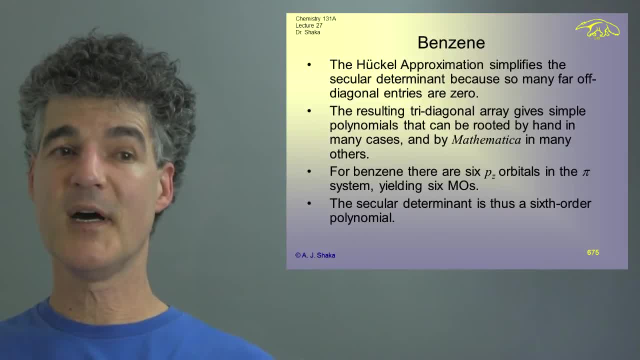 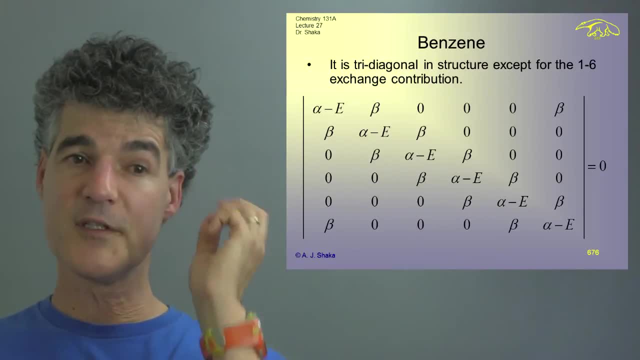 to get our 6 PZ orbitals in the pi system to yield 6 MOs without doing that. Let's set up the determinant then, which I've done here on slide 676 in the Huckel approximation. The nice thing is, except for terms right near the diagonal. 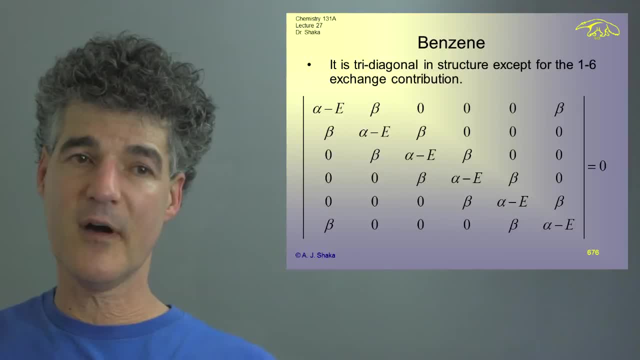 in the array, each of which has beta when they're off, because they all have the same value, and the 6 carbons all have the same integral Integrals for the H11, H22 and so forth. So those are all alpha, and then I have my energy. 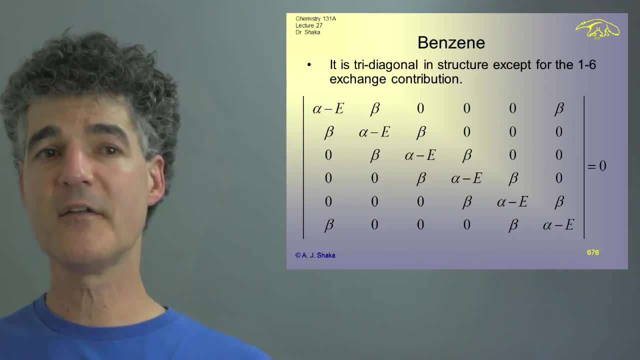 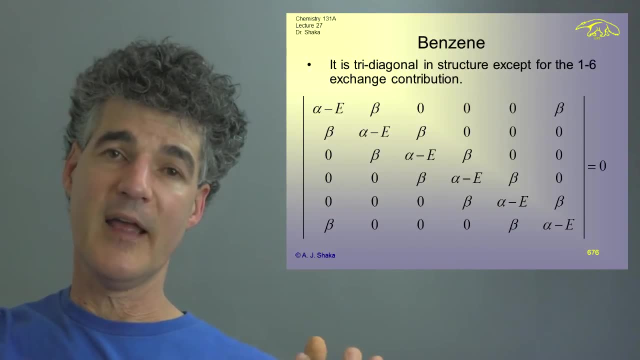 The overlap is gone, so there's no energy off the diagonal. that's very convenient. Everything is zero everywhere, except for the top and bottom, and that's because, as I go around the structure 6 is next to 1.. So you always end up with 1 up there. 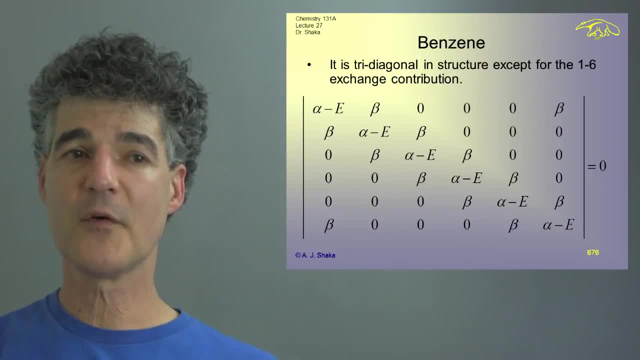 But all the rest are zero, so most of the thing goes away. And we can even make it simpler by, since we've got zero and we know beta is not zero, we can divide everything by beta so that the certain things are 1 if they're off the diagonal. 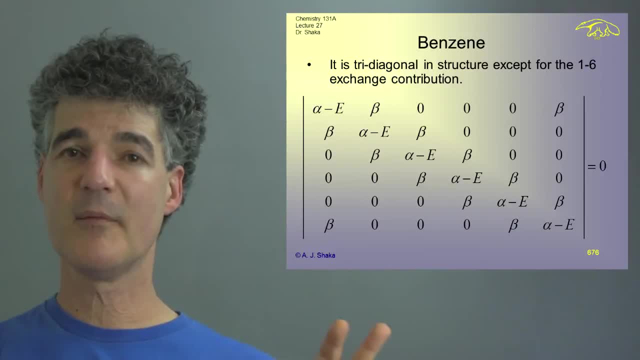 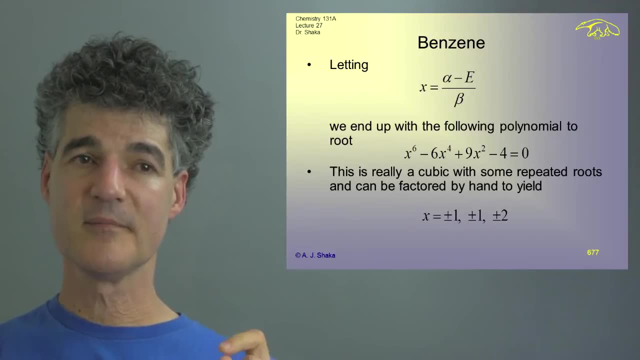 And then we can just redefine alpha minus E divided by beta to be some variable. So let's let X equals to alpha minus E divided by beta, and then all the other terms are 1.. Then we end up with the following polynomial to root: 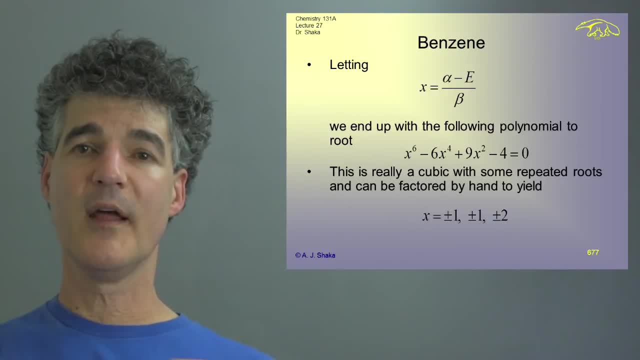 If you expand out the secular determinant, you end up with a 6th order polynomial. It's X to the 6th, minus 6X to the 4th, plus 9X. squared minus 4 equals zero. So that's why you took a course in algebra in high school. 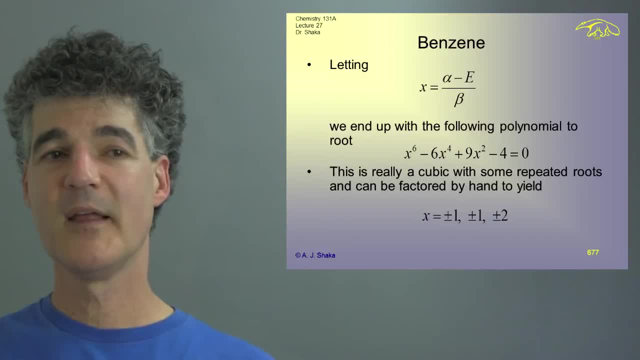 because now this should be a duck soup problem. In fact, it may not be so easy if you just stare at it, but it's not that easy. There's a trick. I'm going to let you explore the trick on the homework, Because it's only even powers we can redefine. Y is equal. 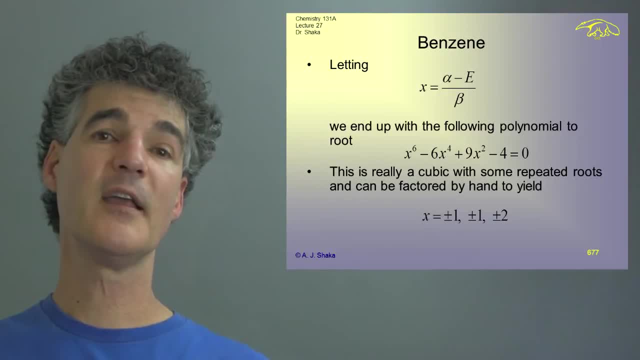 to X squared, and then we've only got a cubic. And if we're lucky we might be able to factorize a cubic and figure out how to actually get the answer. Or we can plot it, even if we're lazy in Mathematica, and we can see where it crosses zero. 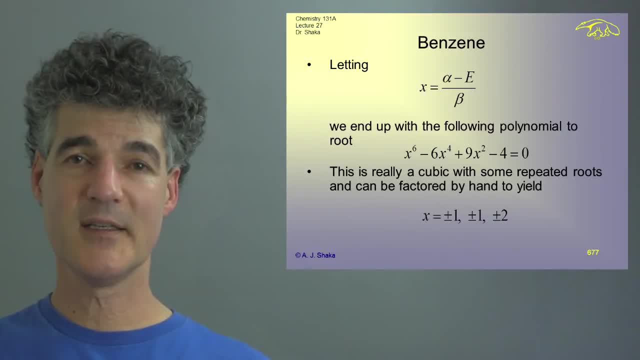 And if it crosses zero at some convenient place, we can get the answer. So that's the trick. If it crosses zero at some convenient place- that is easy to tell because it's an integer- then we can try factorizing it with X minus that integer, X naught or N naught. 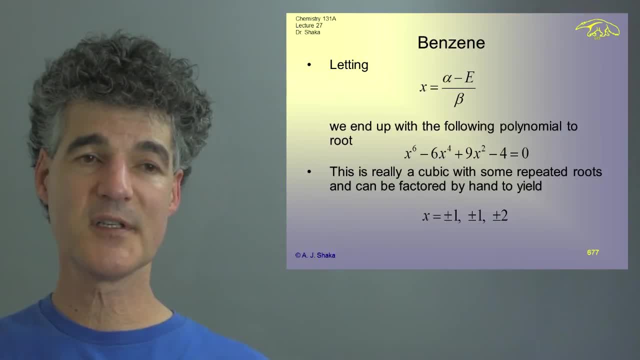 and see if it factorizes. And if you do that and you're persistent, you find that you have repeated roots because of the Y equals X squared, And then some of them are repeated again just because of the structure of what you end up with at the end in the cubic. 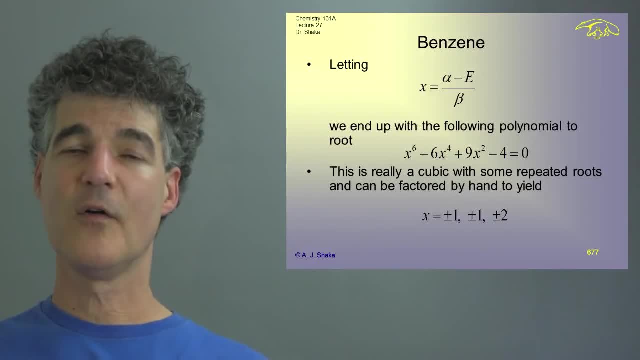 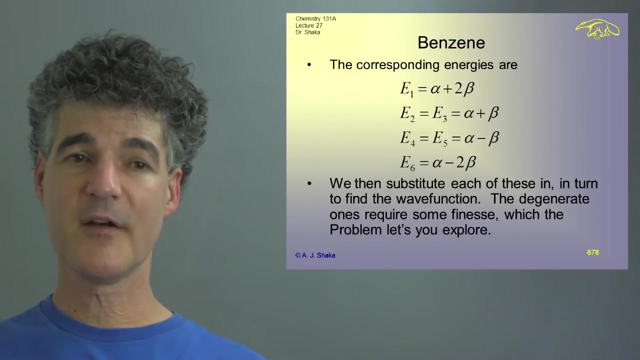 And you end up with: X is equal to plus or minus 1.. Or plus or minus 1. Or plus or minus 2.. Those are the six roots of that equation. Well, X was alpha minus E over beta, And therefore there are the corresponding energies E1,. 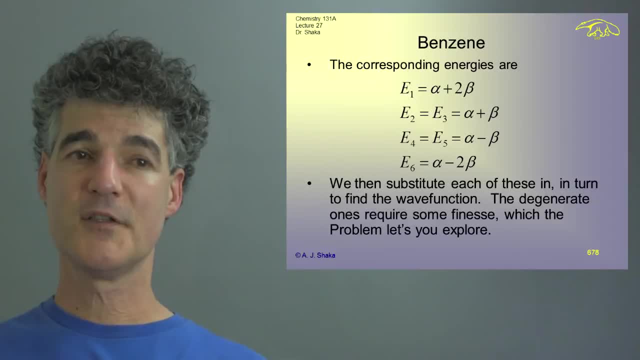 which is the best one: alpha plus 2 beta. Recall that these are usually negative. E2 is equal to E3, is alpha plus beta. E4 is equal to E5. That's alpha minus beta. And then E6 is alpha minus 2 beta. 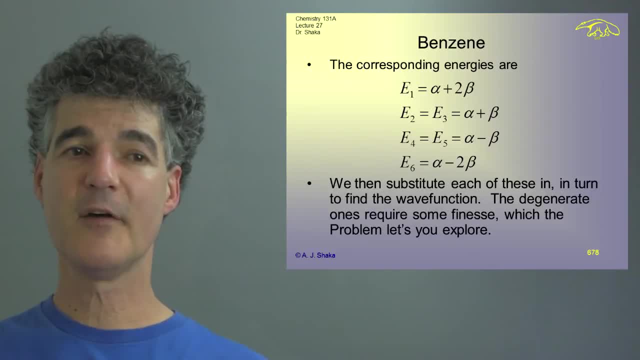 So there's nice symmetry about how the energies come out. Now how do we get what the molecular orbitals are? Recall what we had to do before We go back. We actually put in the energy to the original equation that we had. 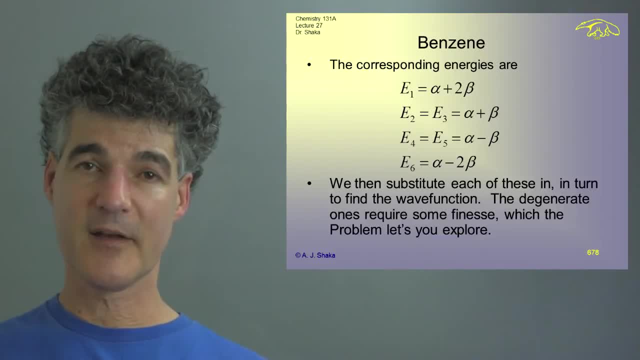 And then we find the orbital that we get that corresponds to that energy. The degenerate ones that have E2 and E3 the same and E4 and E5 the same, require a little bit of thought to how to sort those two out. But whatever orbitals we get, recall that they have. 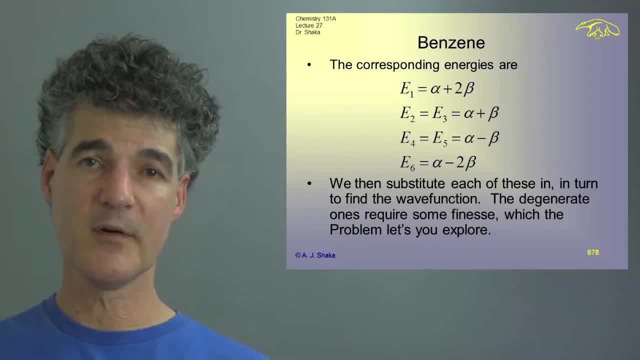 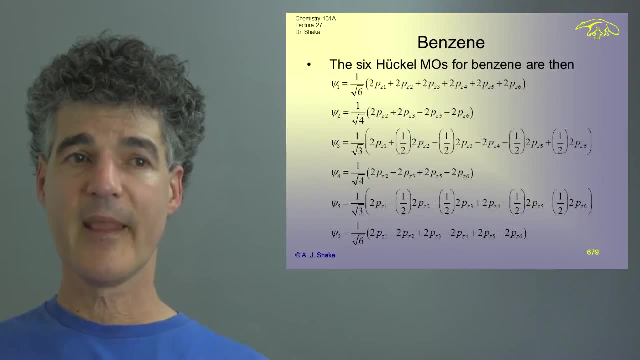 to be orthonormal, The molecular orbitals have to be orthonormal as well, So that's an important thing that lets you simplify it. But I'll let you do that, And here I've given you the answer, The first one, not surprisingly. 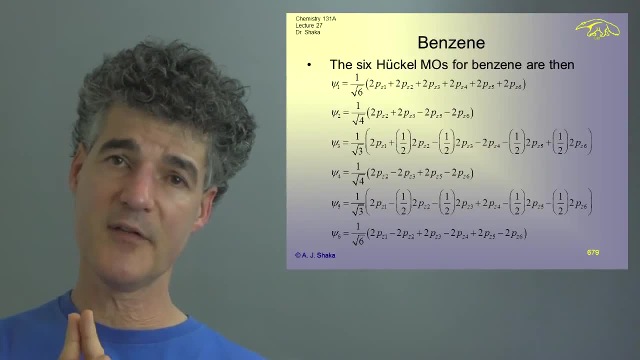 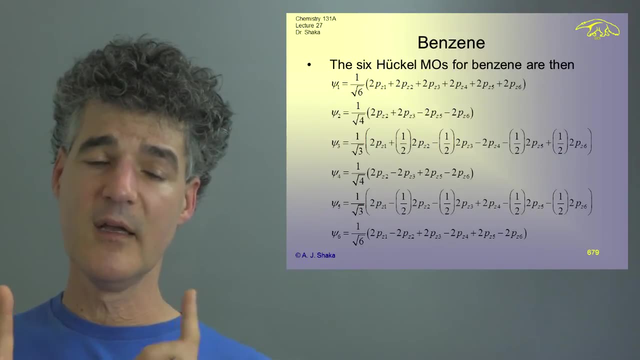 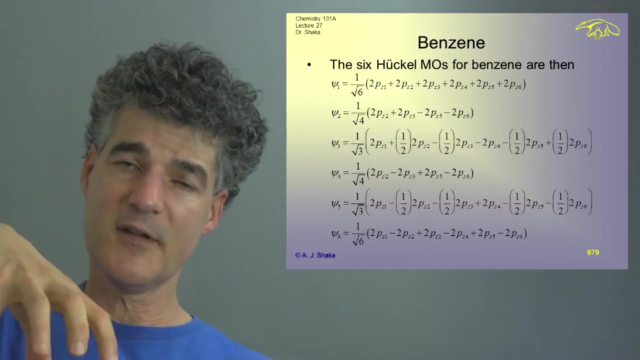 the lowest energy molecular orbital for benzene is when all the six recall benzene is a hexagon planar is when all the six p orbitals have the same phase. So I get a ring of positive electron density around the top. 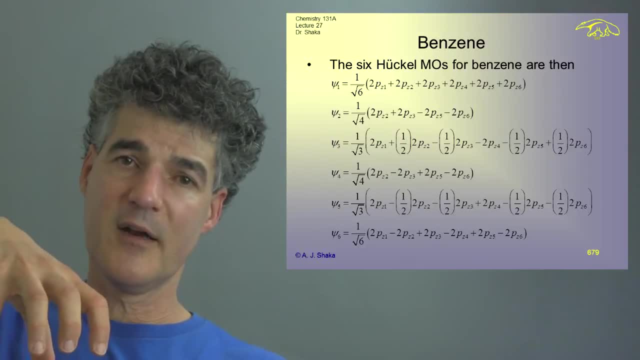 holding all the carbons together And I get a ring around the bottom of the opposite sign. But when I square it I find I build up density And between the carbons, even though they're off axis, and that holds them all together. 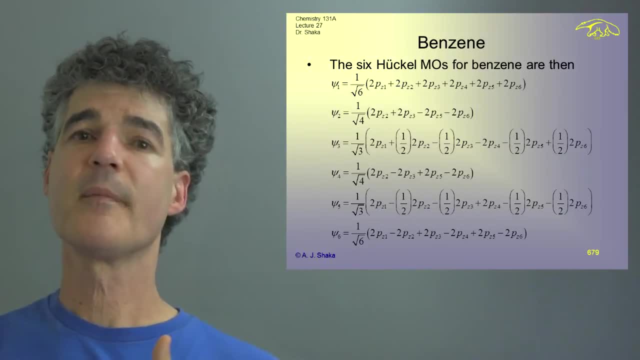 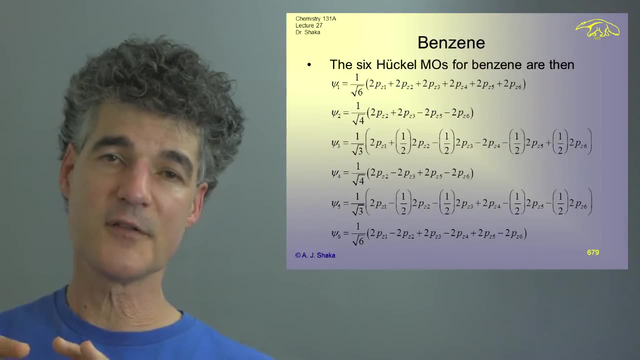 And then the next two have some nodes, but the nodes aren't bad. The nodes are between at certain carbons, And the orbitals are just like methane. They hold the other parts together. So there's one that has a node this way: 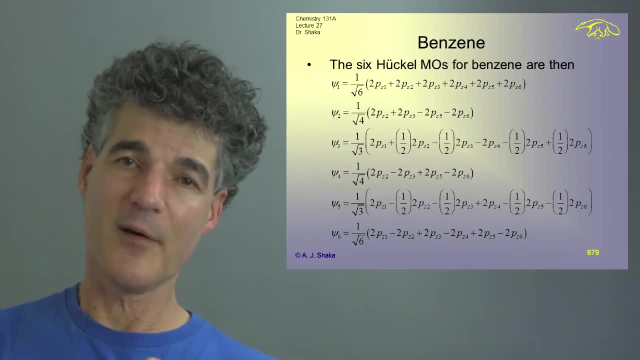 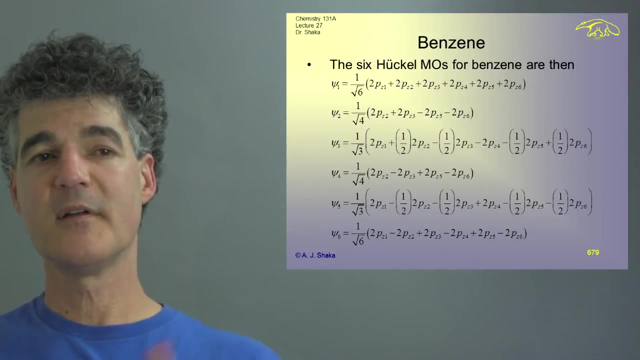 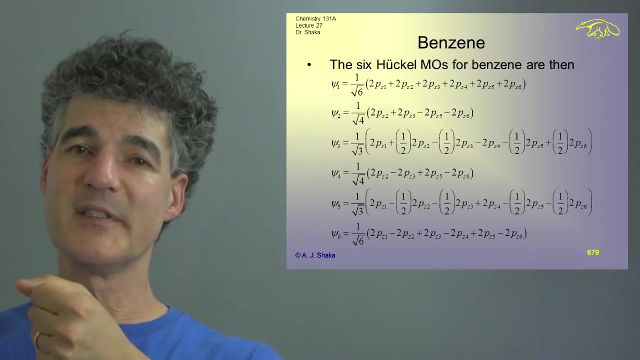 that holds these parts together, And there's one the other way that holds these parts together, And then there's the bad three that have the opposite combinations. basically, And the highest one is when this one's up and this one's down, and this one's up and this one's down, and so forth. 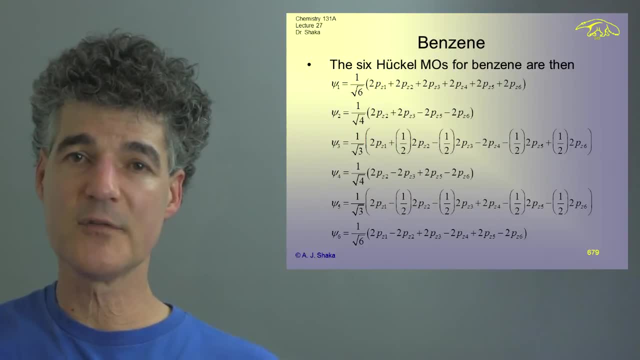 And that has nodes in between everything and tons of nodes, And you can see it's a very crinkled wave function. It's going to have very high energy And that's the least favorable one. That's a strongly anti-bonding. 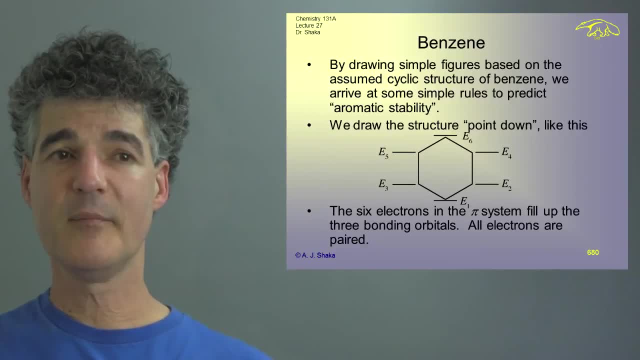 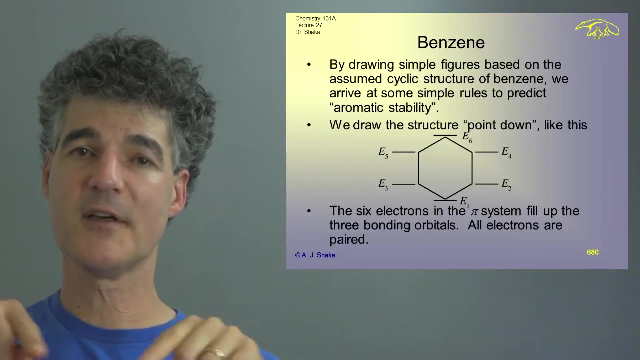 Orbital. And in fact, by drawing simple figures just based on the cyclic structure, you can arrive at some simple rules to predict aromatic stability, You draw the structure point down, And so for a hexagon you draw a point down And then at each vertex you put a line which is an MO. 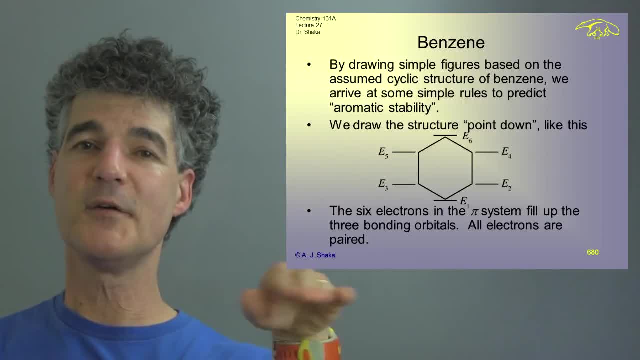 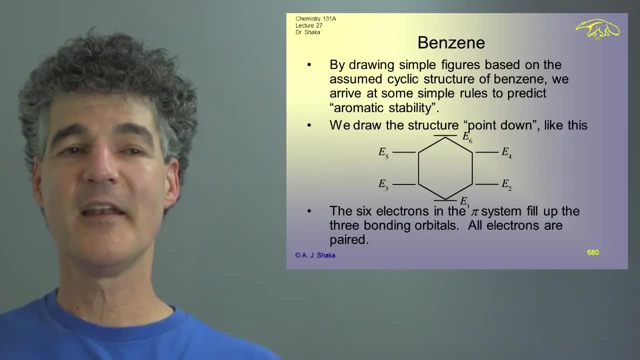 And you have one on the bottom, Then you have two, That's E2 and E3. Then you have these two, That's E4 and E5. And then you have one at the top That's E6. And you've only got six electrons. 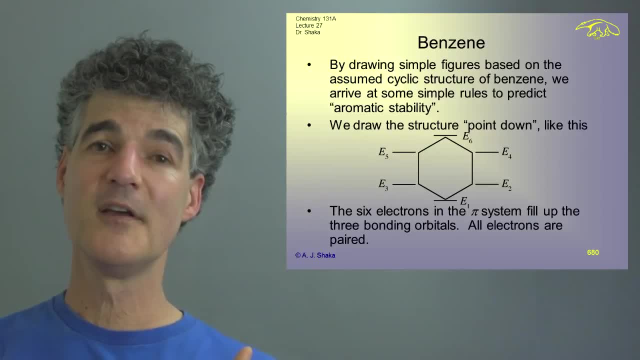 because you only had one electron in each p orbital to start with. So you fill up the bottom to orbital with two, This one with two, This one with two. Game over. So you pick the three good ones, the three winners, And you left all the anti-bonding ones unoccupied. 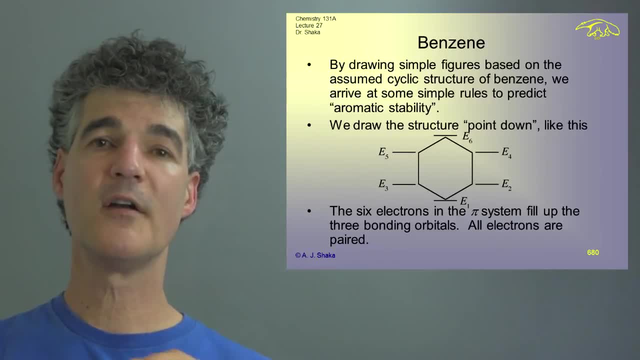 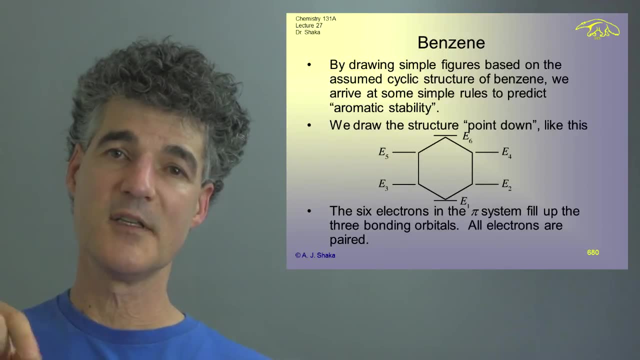 And all the electrons are paired And all these orbitals are delocalized. So we don't predict any difference, Although in the Lewis structure, of course, for benzene we draw a single bond and a double bond because we have to. 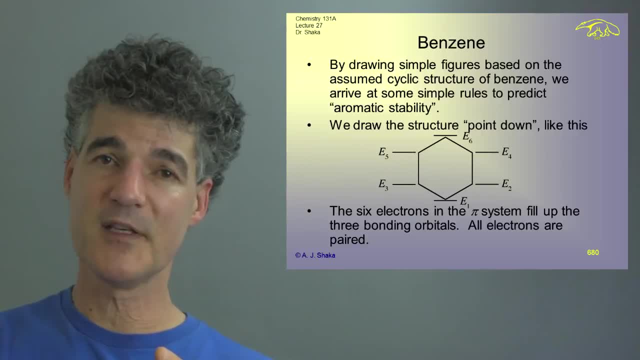 because of the Lewis structure. And then we say, well, there's resonance, We move this here and move them around like a mousetrap In the molecular orbital. we don't have to do that, They're already set up to be delocalized. 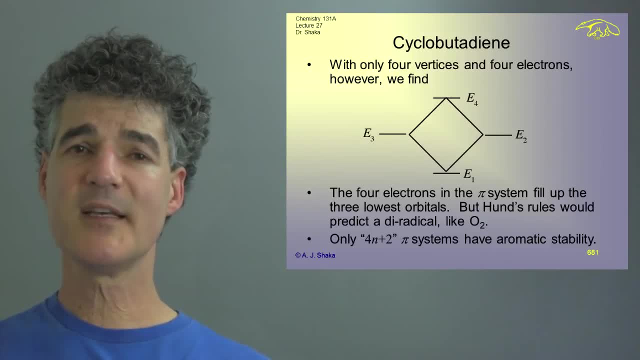 On the other hand, if we pick cyclobutadiene and we stand a square And then we have a single bond on its points, Then we have a lowest one, E1. Then we have E2 and E3. And then we have E4.. 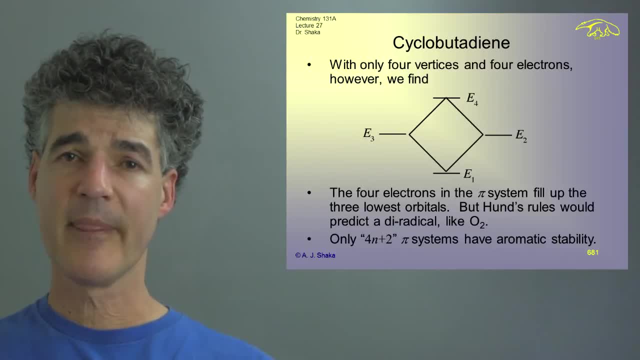 But we have four carbons in cyclobutadiene And therefore we've only got four electrons. So we put two in the bottom, But then we've got two equal ones here. Well, that's like O2 again. So one goes here and one goes there. 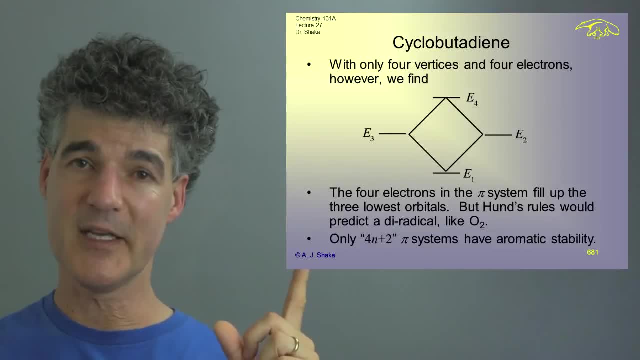 Well, that's not aromatic. That's not aromatic, That's aromatic stability. That's predicting a di-radical. I wouldn't take this kind of very qualitative thing too seriously. I'd do some spectroscopy to figure out what you actually get. 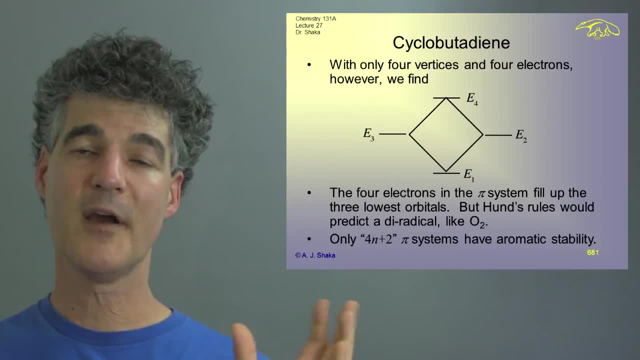 But whenever it comes out like that, where the two aren't paired and there's some left, the conclusion is it's not aromatic. And what happens then is the ones that have 4N plus 2, pi N plus 2.. pi electrons become stable. 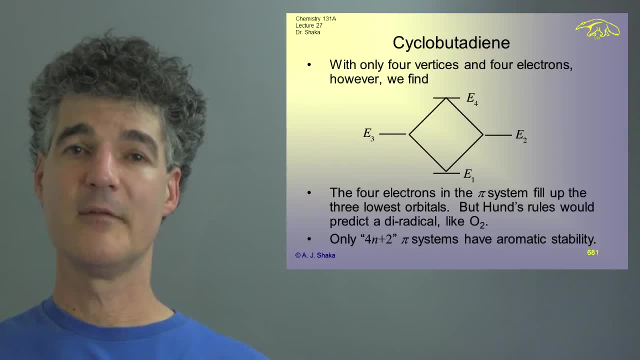 And the ones with 4N, like 4 rather than 6, are not especially stable, and not stable at all in some cases. So only the 4N plus 2 pi systems are predicted to have aromatic stability, And that comes out of a more detailed calculation too. 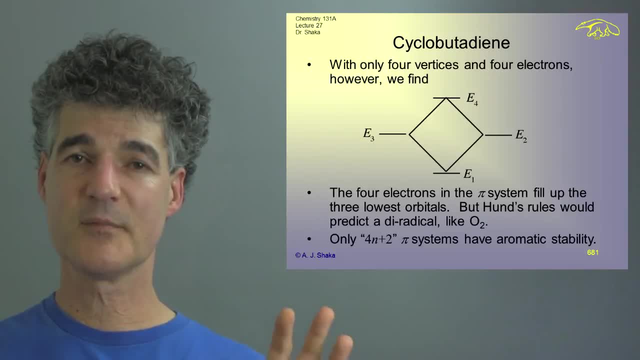 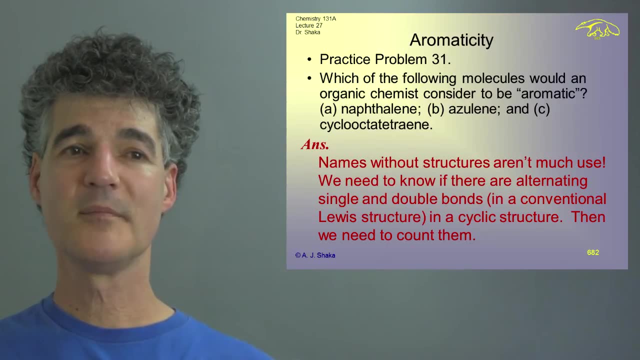 not just playing games with shapes. But it's interesting to just play games with shapes because it's very quick And often it's good enough. All right, let's do a practice problem. Let's consider the following molecules and let's consider them. 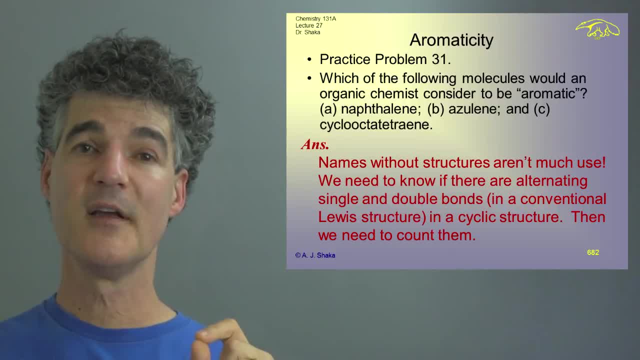 and see which ones an organic chemist would predict to be aromatic. so they have this special stability. Benzene was used as a solvent for a long time. Why? Because it doesn't react with anything, So it's a perfect solvent If things won't dissolve in water. 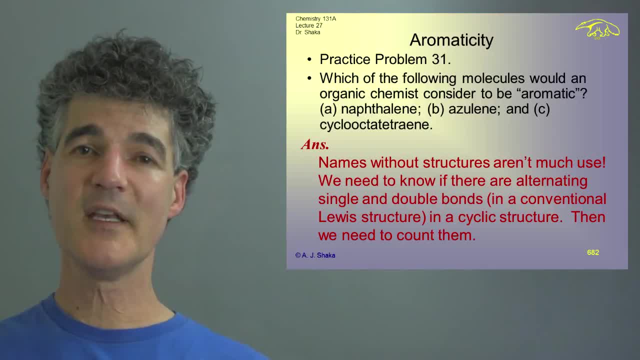 or they're reacting with anything, it's a perfect solvent. If things won't dissolve in water or they're reacting with anything, it's a perfect solvent. If the reaction is slow in water, you dissolve it in benzene and the reaction goes very quickly. 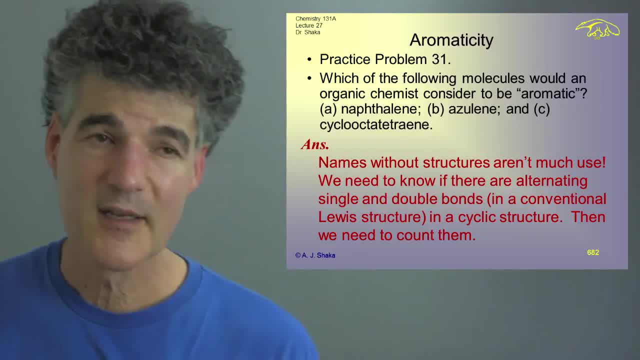 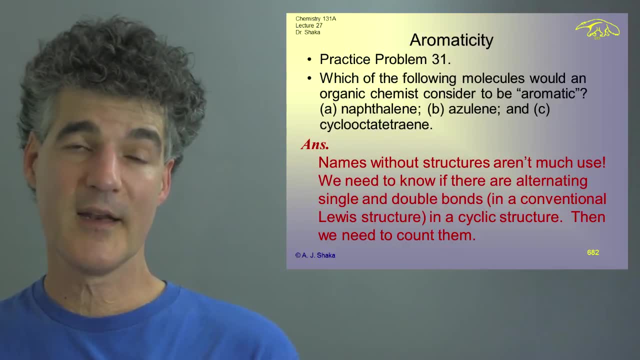 The problem was, of course, benzene is quite a potent carcinogen, like a lot of these systems, and so if you're breathing a lot of it and boiling it up and breathing it on a daily basis, it's not the greatest, and that's why they went away from it. 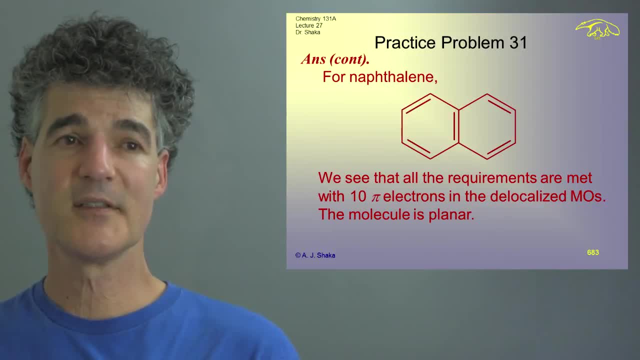 Let's consider then benzene, we know is aromatic. Let's consider naphthalene, which is in mothballs, That's that smell. Azulene, which you probably haven't seen nor smelled, and then cyclooctatetraene. Let's take these three and see what they are. 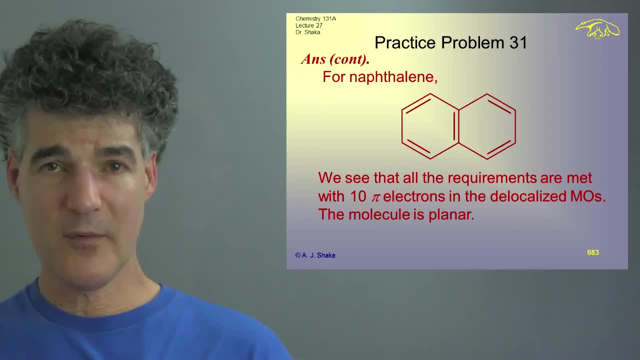 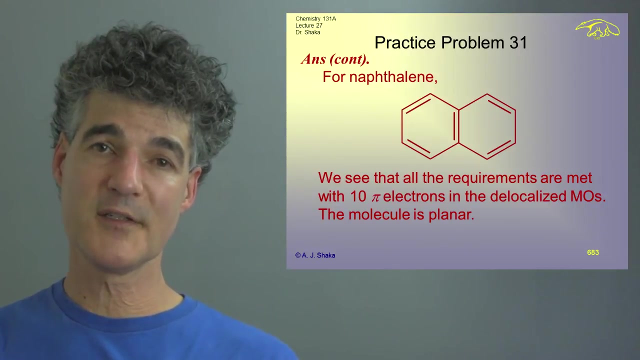 Well, first thing is the names. if you don't know what the structures are referring to, the names are useless and we have to know they aren't going to be aromatic unless in the Lewis structure they would have alternating single and double bonds and we could do resonance. 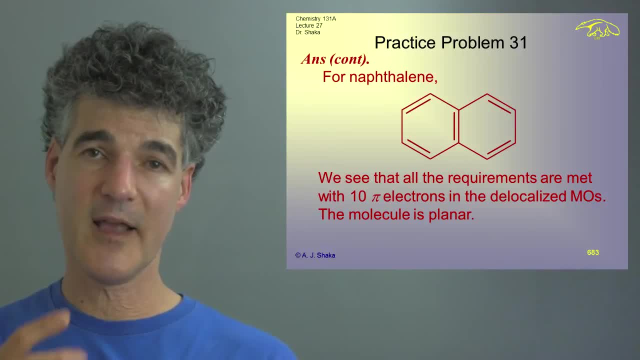 and move the things around so that they would all be equivalent, half the time single, half the time double. If they aren't even like that, then forget it. It's not going to be an aromatic system, or the part that can't do that trick with resonance is not going. 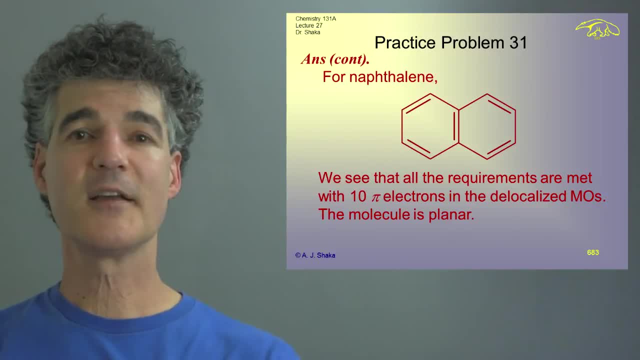 to be an aromatic system And they have to have a cyclic structure as well, so that the snake bites its tail, because that's important in how those two last terms come in. If those don't come in, a lot of things change, it turns out. 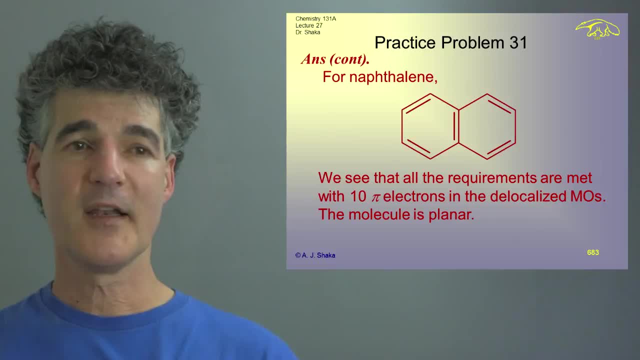 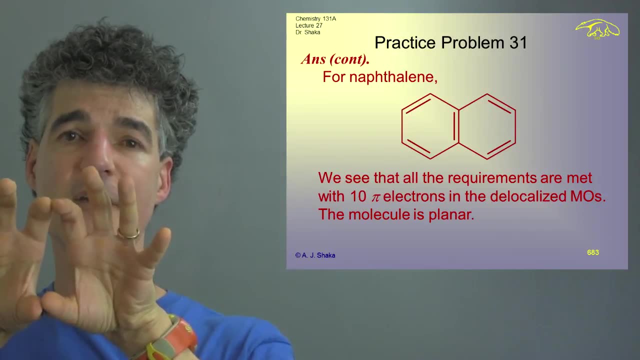 And then let's draw the structures and count them. So for naphthalene we've got two benzene rings fused together. Now if we were actually going to do the MO treatment, we'd have to be careful, because these two carbons 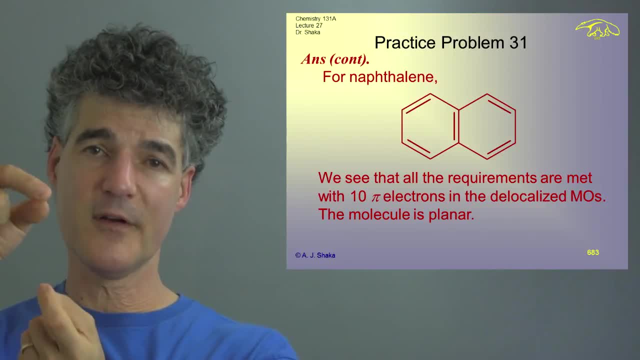 without any hydrogens on, could have a different coulomb integral than the others, and the others would all be the same, and so we should take that into account. We should have alpha 1 and alpha 2.. If we're lazy, we just say well. 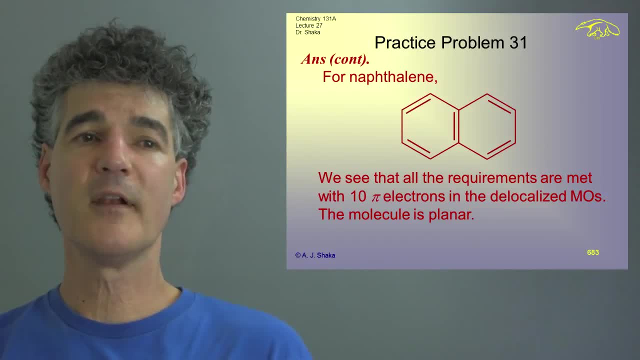 they're about the same. call them alpha, And I've drawn the Lewis structure here, one of them, and we could play a game with resonance then and draw one the other way. We count the electrons in the pi system. We forget about the sigma. 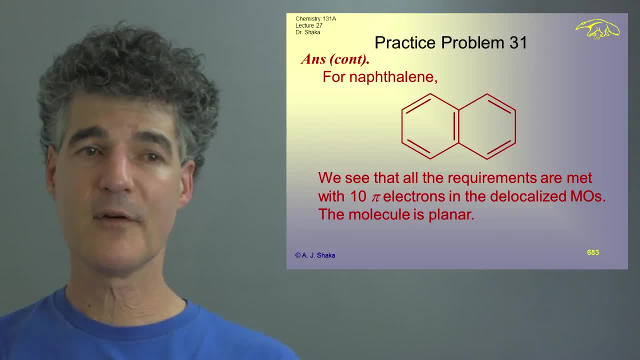 We forget about the hydrogen and we see there's 1,, 2,, 3,, 4,, 5,, 6,, 7,, 8,, 9, 10.. That's 4n plus 2 for n equals 2.. 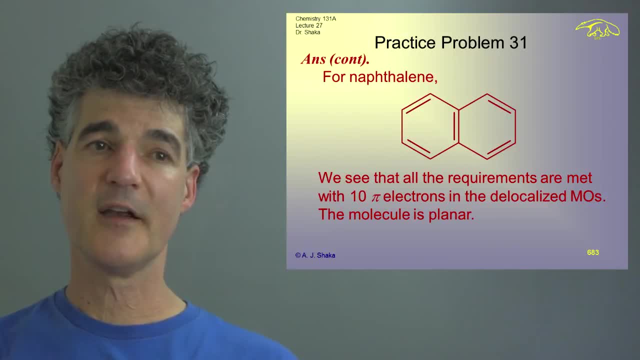 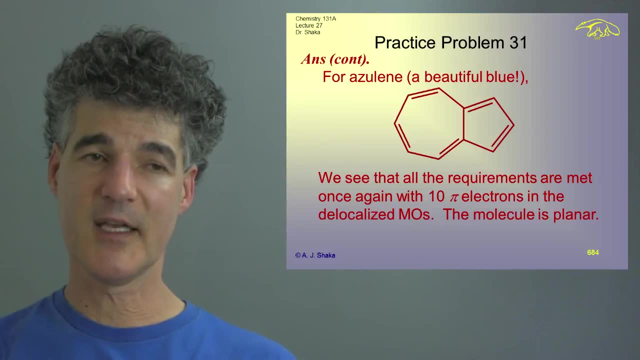 And so it's planar and it is, in fact, aromatic For azulene, which is a structural isomer of naphthalene. there's a 7-membered ring glued to a 5-membered ring And I can still draw the double bonds the same way. 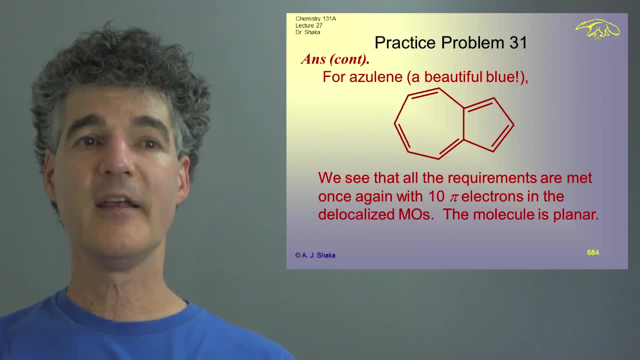 It's kind of amazing that it works like that And it's a beautiful blue color. And again, I count up: It's a cyclic system. I count up: There's 10 pi electrons and the delocalized MOs go over the whole thing and it's planar and it's very nice. 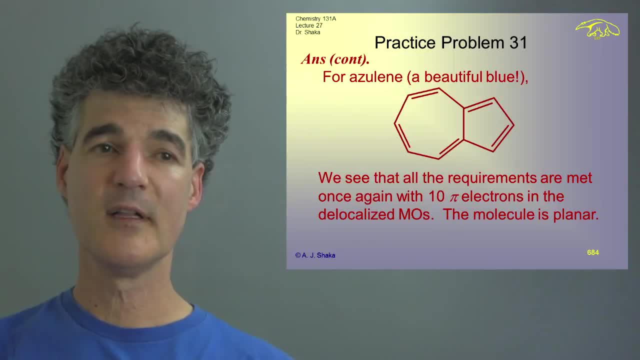 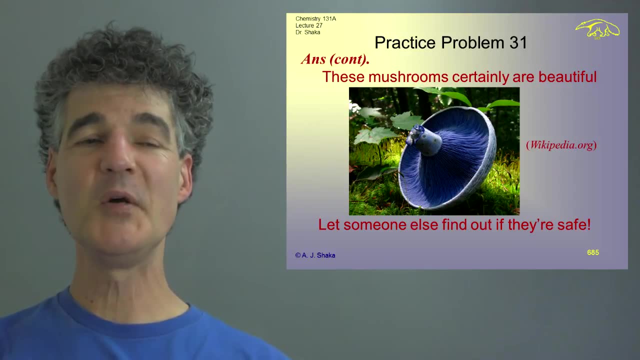 an example of an aromatic system that's not so trivial, like a benzene one. And then here, what I've shown you is a mushroom that is blue. It's absolutely amazing, But in fact this mushroom makes an azulene, and it's a very interesting derivative. for some reason, 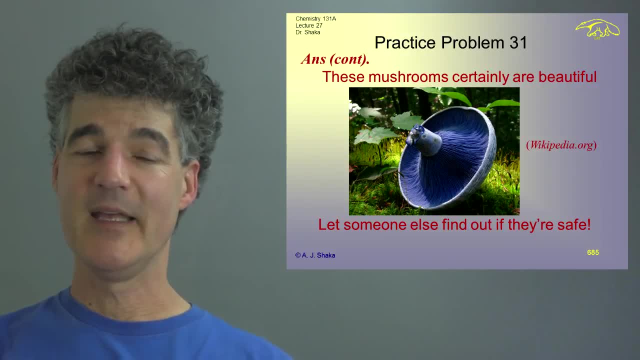 probably extremely interesting chemistry. Usually, when plants make interesting molecules, it's because they're keeping bugs off or keeping other things away, Because too bad for plants. they can't move And if you're stuck and bugs are crawling all over you.